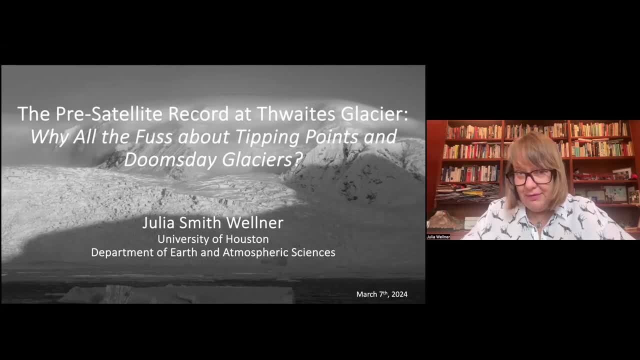 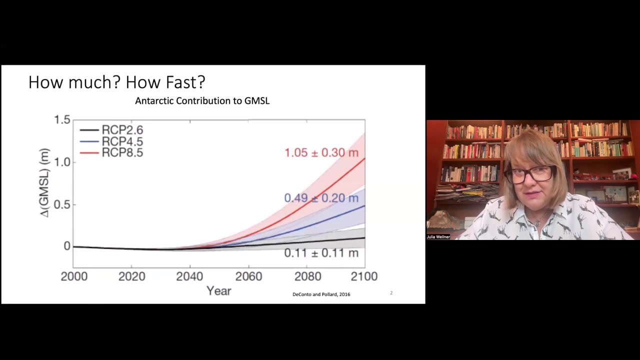 as part of the current international Thwaites Glacier collaboration, And I'm going to show you the part that I do lead. So, to get started, I just want to give a very brief background about why we are interested in Thwaites And of course that is based on concerns about future sea level. Many of you may know this. 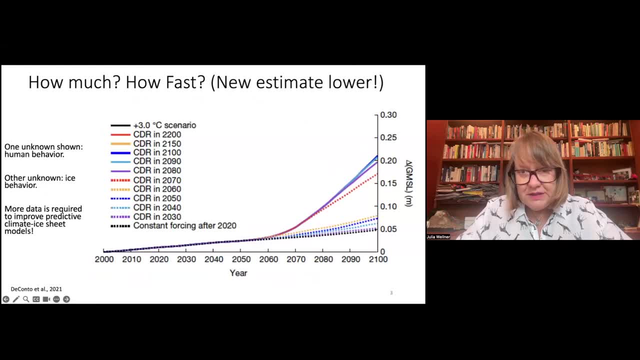 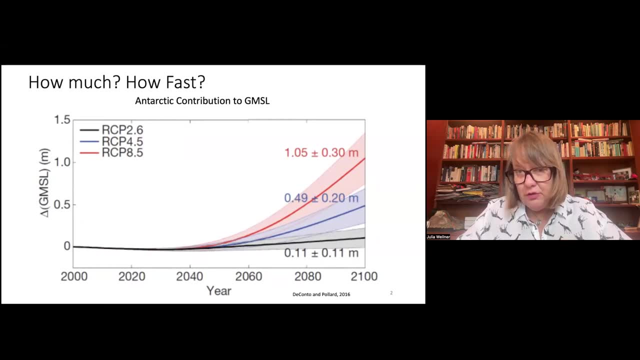 curve, which is- excuse me- from 2016, and predicts just the potential contribution to global mean sea level that might come from Antarctica. So this is not the total potential sea level rise, but what might be contributed to global change from Antarctica. 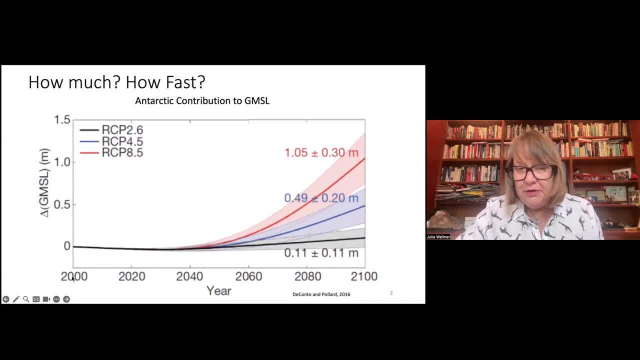 And on the x-axis we have time going from the year 2000 out one century, And on the y-axis is the potential increase in sea level from nothing to a meter or more, And what you can see on the slide is that there's a huge range. I'm not going to talk through all of the ambiguities in these. 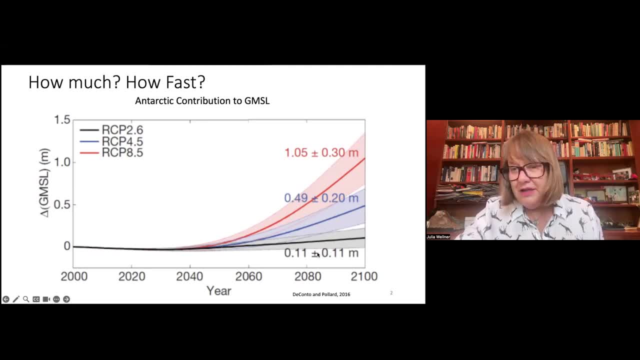 different numbers, but what we can see is that it goes from nothing to about a meter or more, And that means that we, even just a few years ago, didn't have a clear understanding of what Antarctica might do In an update to that paper. so these are the same authors, largely. 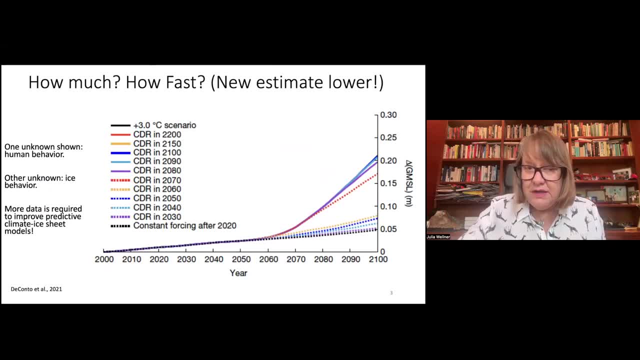 but with a paper from now, just three years ago- 2021,, we see the same setup, with time on the bottom axis going out one century, And then Antarctica's contribution to global mean sea level, And, of course, these are different emissions scenarios, And what we see is that there's a lot. 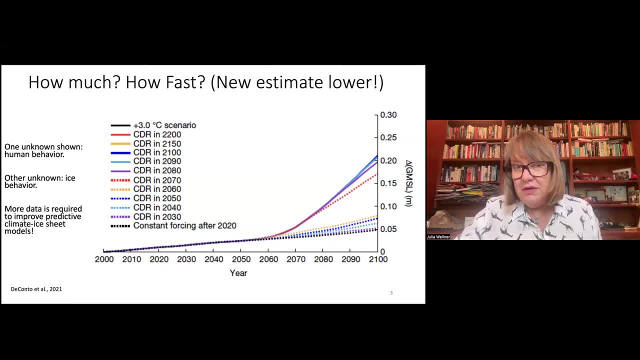 of unknowns in emissions scenario, but we also have unknowns in the ice behavior, And so the purpose of the International Thwaites Glacier Collaboration is to better understand how ice is behaving today and in the past, so that we can understand what it might do in the future. 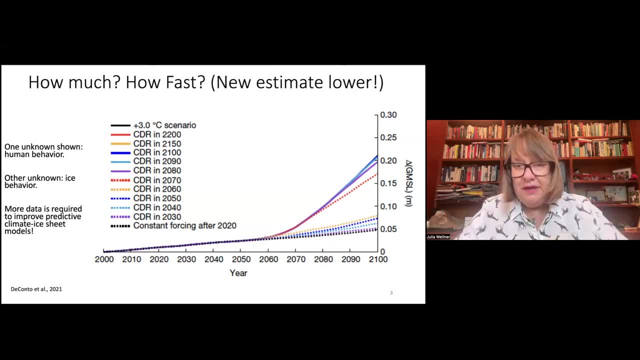 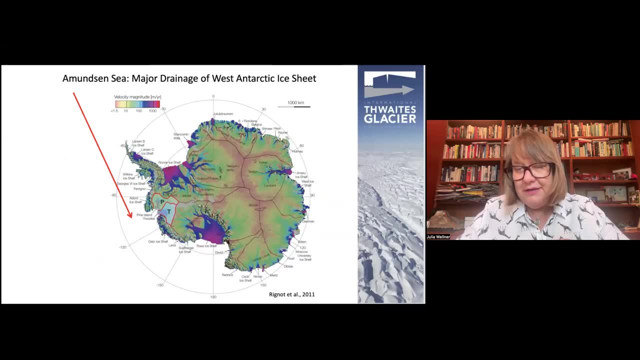 Let's constrain these models down a little bit to make better predictions, not just about people, but about ice. So the area we're studying- I know this is a primarily Arctic group, but I'm sure you're familiar with the Antarctic as well. 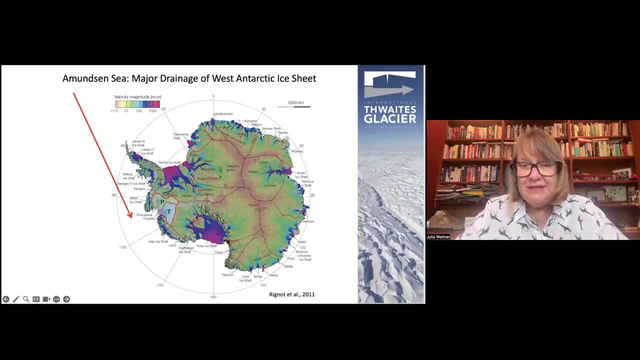 And so this part of Antarctica is West Antarctica, and in the middle of West Antarctica is the Pine Island and Thwaites Glacier embayments that drain into the Amundsen Sea. Pine Island and Thwaites Glacier are in the news a lot because they are both rapidly changing and large drainage basins. 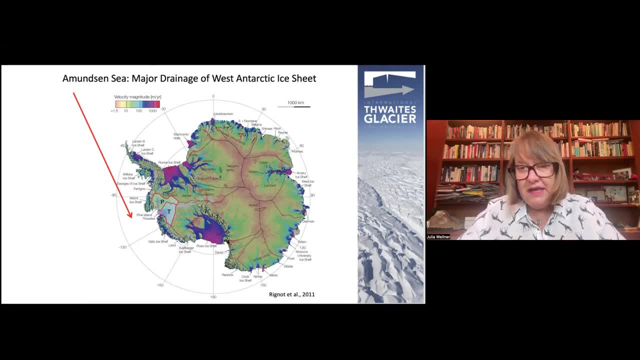 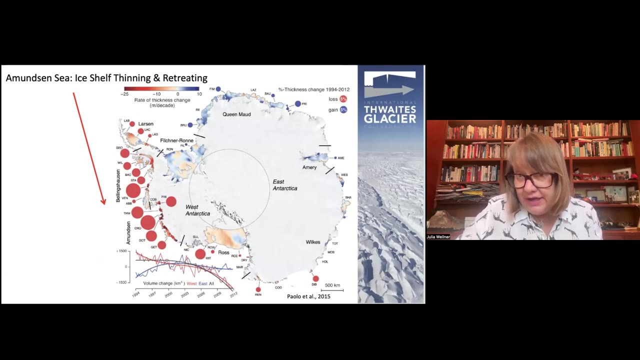 And so in this image we're looking at ice velocity and you can see that the ice is flowing rapidly in a few of these major embayments, including Alonson Sea. And in another image of understanding how ice has changed over recent decades, we can look at the red dots that indicate ice shelf thinning and retreating, where the scale of the dot represents the amount of change. 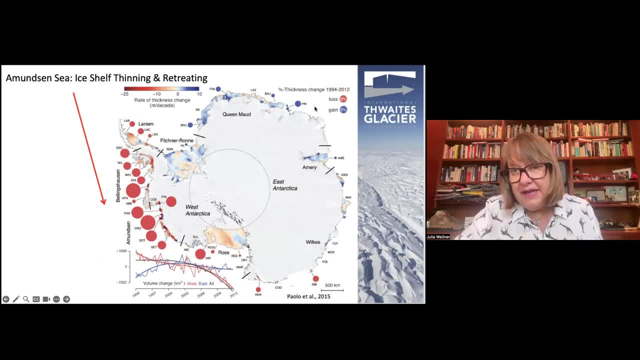 And then there's also some blue dots over here that indicate thickening and advance. What we can see is that the ice has changed, And what we can see quite easily is that there's lots of big red dots around the Thwaites Glacier area, indicating that it is rapidly changing. 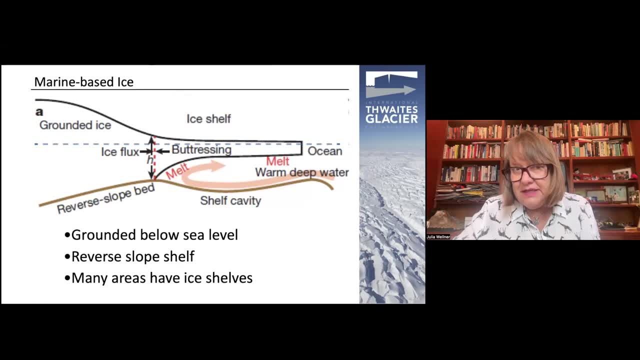 The reason that Thwaites is of such interest is that it is a marine-based glacier. Marine-based ice is susceptible to rapid change for a variety of reasons. The three main reasons are that that ice that's Sitting in the ocean is obviously sitting next to something that is warmer than ice. 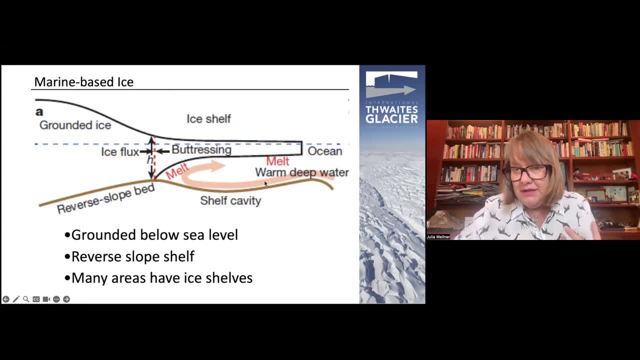 This liquid water in the ocean is warmer than the ice And in Thwaites in particular, we have warm deep water that's flowing in and reaching the base of the ice, which can melt the ice at its base. In addition, Thwaites Glacier, like other glaciers, is a very warm deep water. 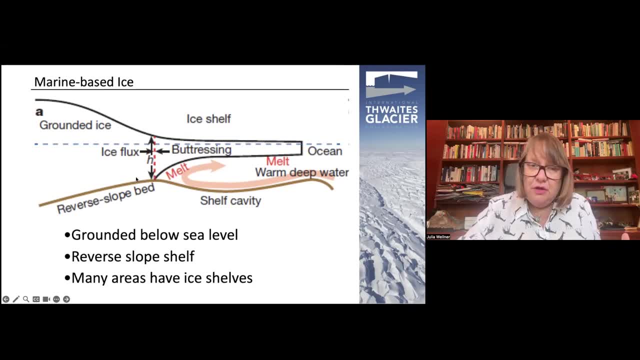 And, of course, the ice that's floating in the ocean, which is known as the ocean's surface in West Antarctica, sits on a reverse slope bed, And that's shown in this cartoon right here. That reverse slope bed means that once the ice starts to step back, it loses its footing. 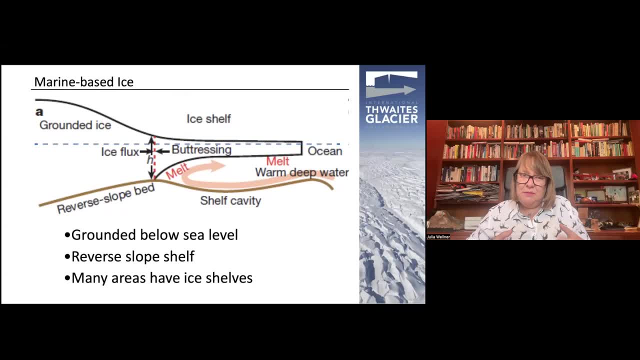 And it's even harder to reground and even harder to get its stability again. And then, lastly, marine-based ice, including Thwaites, has an ice shelf. An ice shelf is already floating and therefore won't add to global sea level should they melt or decay. they do serve as a buttress to the ice. 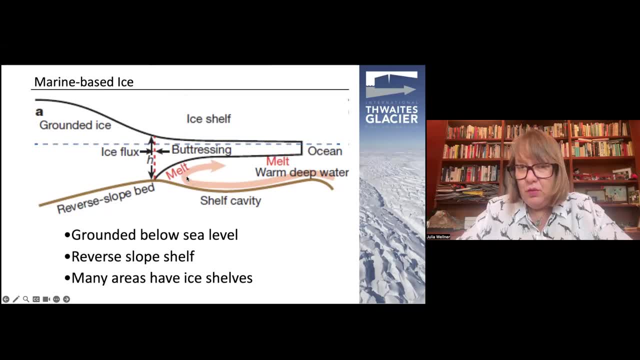 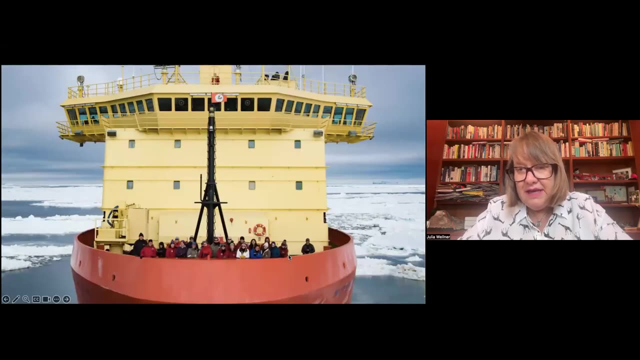 behind it. And so all three of those things- the warm water, the reverse bed and the ice shelf buttressing what's behind it- make Thwaites susceptible to rapid change. So I am representing a project that has had a series of field seasons on the Nathaniel Palmer, which is an icebreaker. 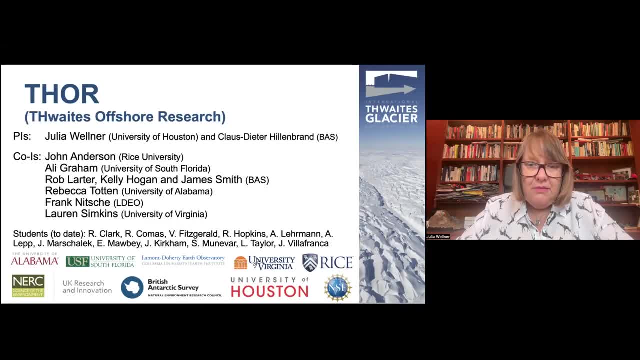 operated by the National Science Foundation. This is a project called THOR, which just stands for Thwaites, Offshore Research, And you know in Pam's introduction she said that I was leading part of this and this is a component. We have about 10 US universities. 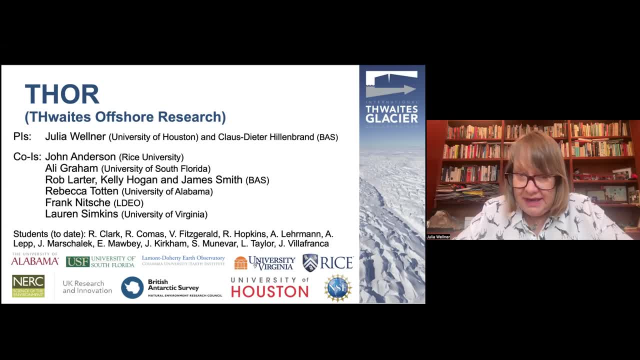 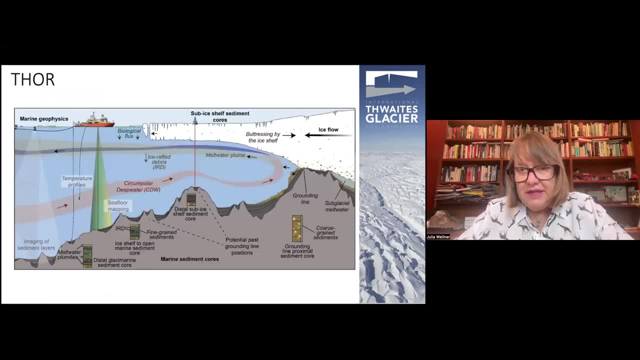 involved, as well as a few in the UK and the British Antarctic Survey. THOR is a project aimed at understanding Thwaites Glacier from the marine margin In Antarctica, of course, where it's relatively cold in the air. we're not thinking about ice, shelf melt or ice. 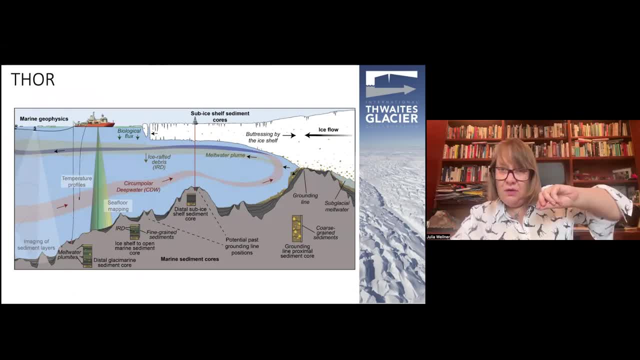 melt from the surface where the air remains relatively cold. So really to understand what's drastic- and we have to do some work on that, And so we would like to talk about that for a bit. So in the last slide we have the NAVARNRAN, whom is a great resource for these surveys, which includes 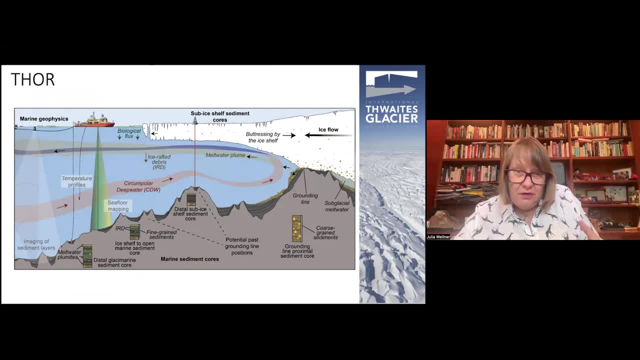 driving change in the ice. we need to think about the ocean-ice interface. We approach that from two ways as part of this project. One is from the icebreaker. Here's the cartoon of the Palmer showing us collecting geophysical data, oceanographic data, sonar data. We also collect 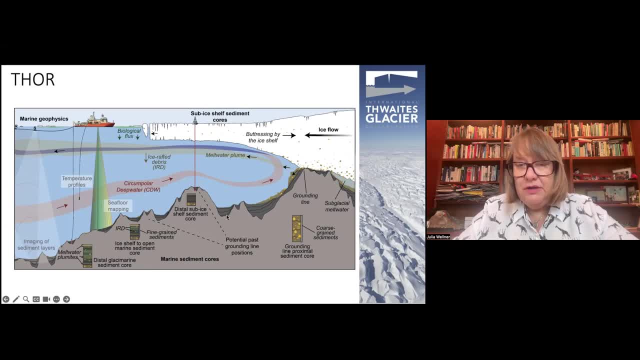 these sediment cores which are shown down here and I'm going to show you in the coming slides, And our project does also work to collect sediment cores through that floating ice shelf. I'm going to start with a little bit of extra high-resolution data, though. 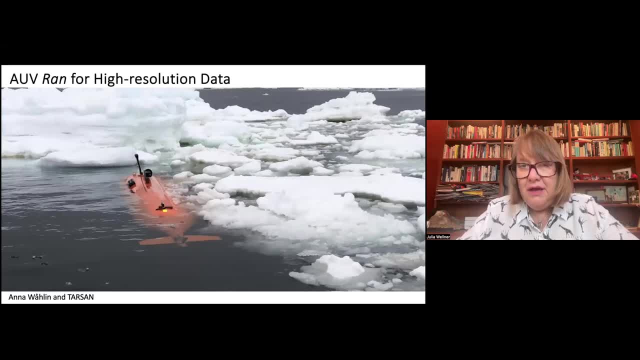 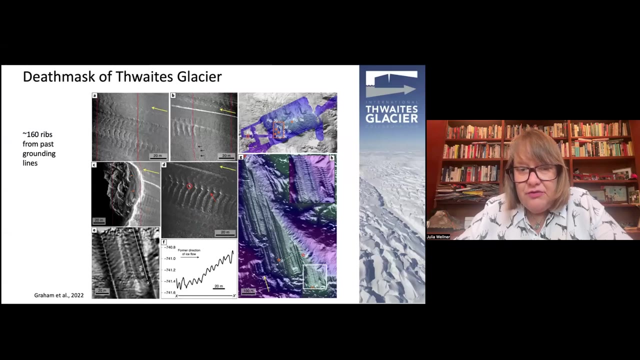 and this is actually collected from an AUV from Huginn, and this data gets down closer to the seafloor and therefore allows us that extra high resolution. So I'm starting with a paper that was published a year and a half ago. 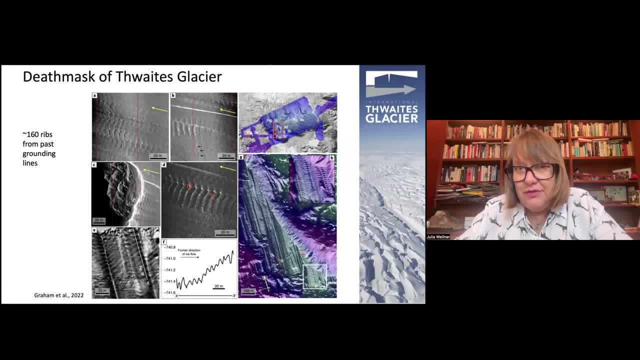 It's showing the death mask of the Thwaites Glacier. What do we mean by death mask? The imprint of what was left behind the last gasp of when the ice was sitting on the seafloor and what that recorded. And in the colored image on the right you can see some great long lineations Those show the direction of ice flow over time. 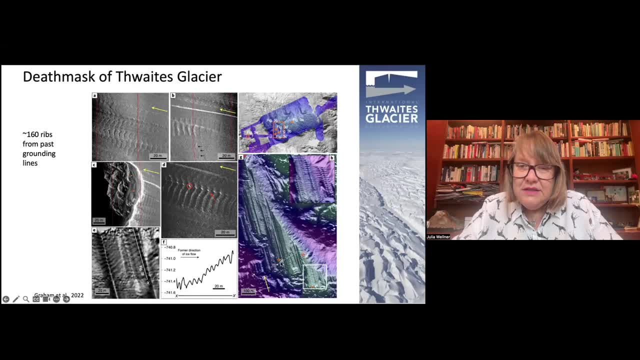 But within those lineations you can see some ribs and these ribs are shown here in this side scan sonar data, which is like an aerial image of the seafloor. It almost looks fake but because those images show us the individual spots where ice has grounded in the past. that forms by ice sitting on the seafloor and building the seafloor around it. 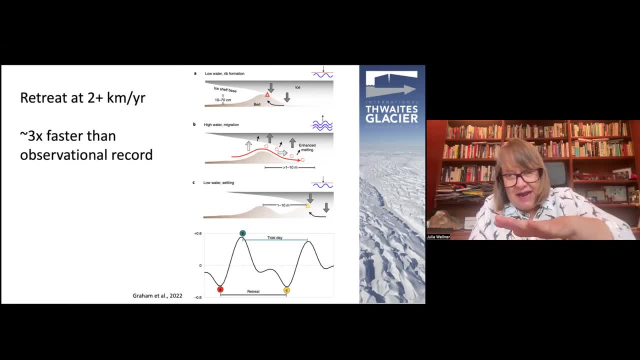 sort of moving up and down with the tides as the ice pulls back. So during retreat each rib represents a tidal cycle. So we can count that distance and that shows us a retreat of around two kilometers per year, which is about three. 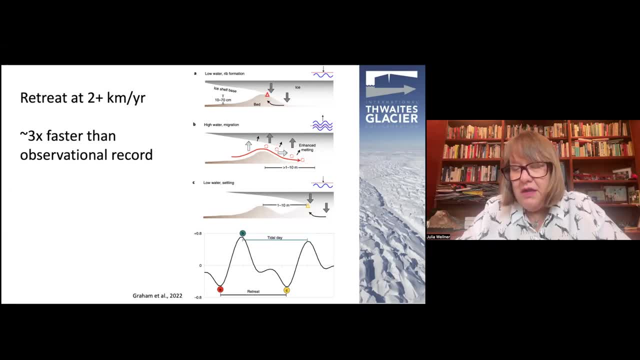 times faster than the observational record today. Now, this maybe didn't last long, It may be didn't make a significant contribution to global sea level. We're not showing that this happened for the entire retreat, but rather just that that speed of retreat is possible three times faster. 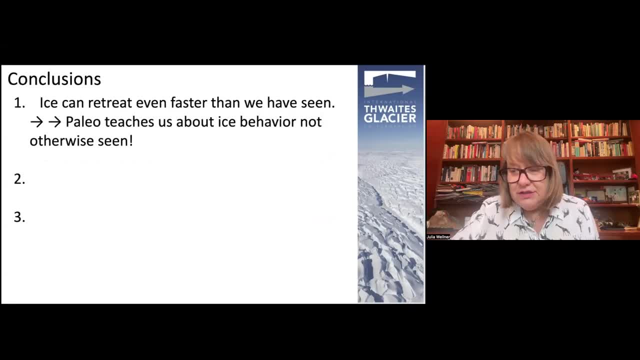 than yet observed, And so I have three conclusions for you today. That's the first one: that ice can retreat even faster than we have seen, and that paleo records- the geologic record- teaches us about ice behavior That's not otherwise seen. My specialty is working on sediment cores, and we collect a. 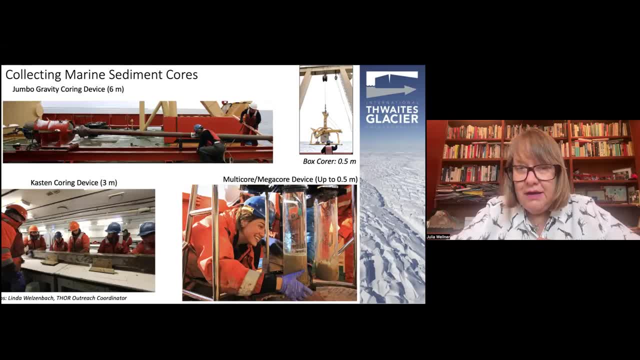 variety of types of sediment cores in the Antarctic. We take these very long cores called jumbo piston cores. We take medium length, called casting cores, and you can see all of us carrying it indoors here to work on it. And then we take these very short cores so that we get really 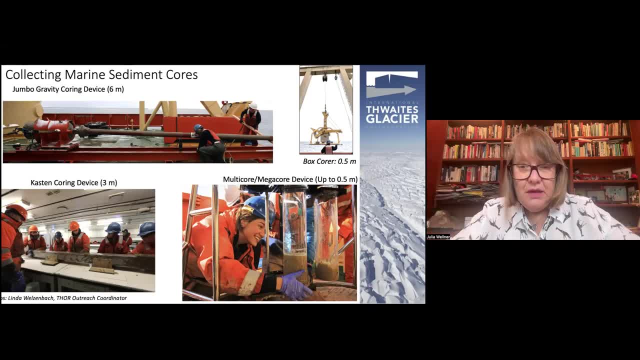 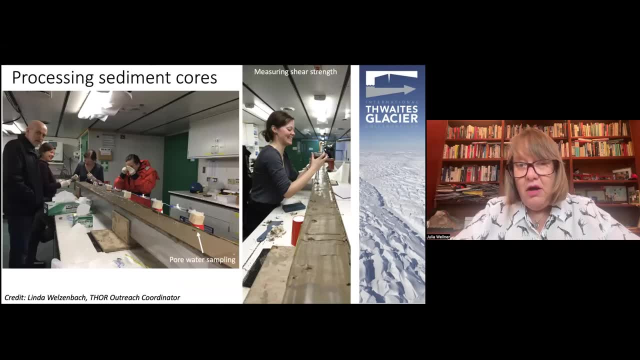 pristine, clean records of the recent history. We bring them into the labs on the ship. We do a variety of analyses immediately on ephemeral properties that will change. That includes things like shear strength right here, pore water sampling, where we actually get the water out to do chemistry. 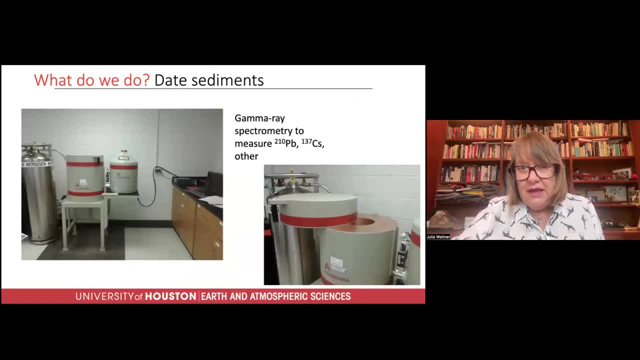 before anything changes, And these are a couple pictures of my lab at the University of Houston. This is a gamma ray spectrometry system. This is 4,000 pounds of lead shielding, not to protect any samples that I have that are radioactive, but to prevent any radioactive air or 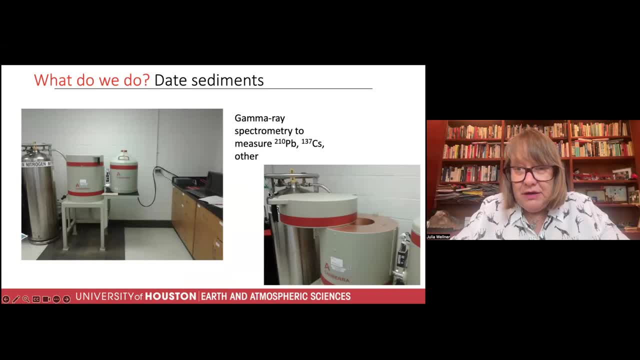 dust from getting into the measurements because we are measuring such low levels of radioactivity in this gamma ray decay And I'm dating both lead to 10 ages and sometimes cesium 137. And that's what's really highlighted in this paper that Pam asked me to show you. 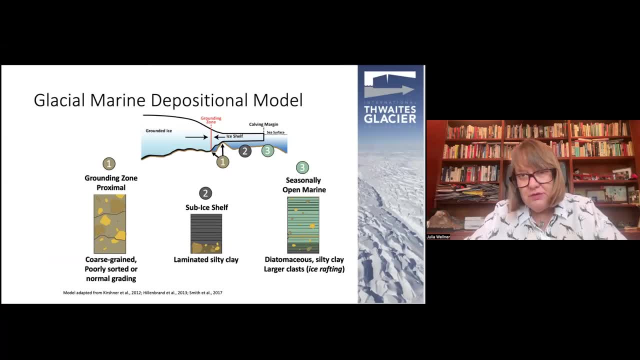 And a glacial marine depositional model that shows how ice has retreated over time. Because we're working in the ocean, some of what we're recording is marine sediments, But because the ice has retreated back over time at the interaction between the ice and the ocean from a position that is now ocean. 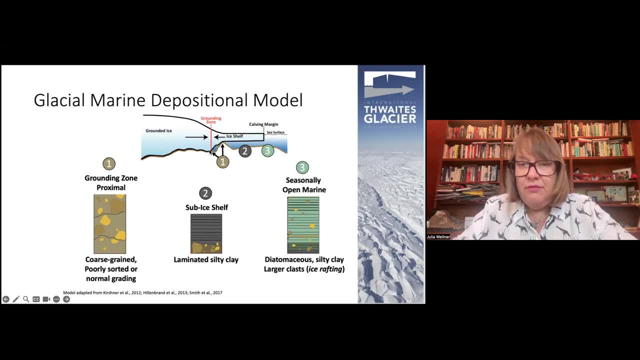 And so the first faces that we look at might be from this grounding zone or where the ice is pinned in the ocean, and those sediments are very coarse, they are unsorted, possibly a little bit of grating, but not much, and they tend to be stiff or have high shear strengths. 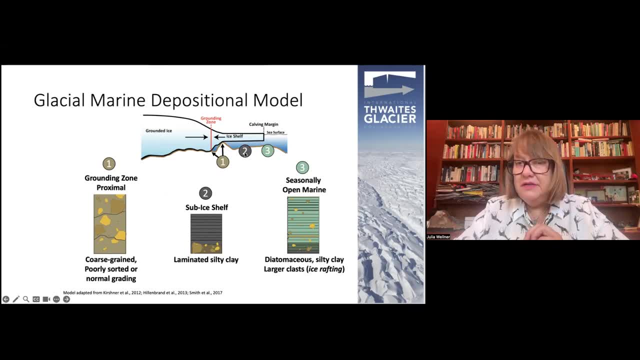 In Zone 2, shown here underneath the ice shelf, we get limited deposition because it's not receiving much sediment from the ice or from the ocean, sort of this null zone in between. In that case we get very slowly accumulating laminated silty clays. 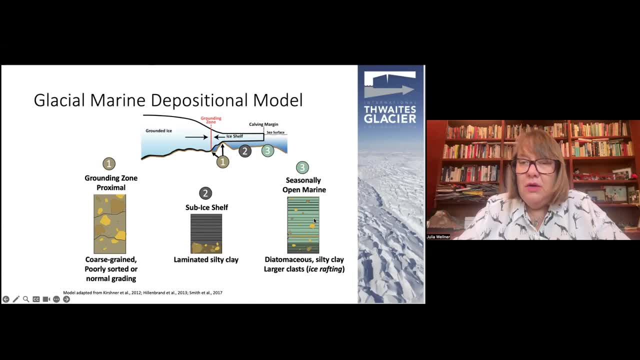 And then out here in Zone 3, in the open ocean- or at least seasonally open ocean, depending on the sea ice- we get diatomaceous sediments, which is diatoms are phytoplankton, So this is a biological deposit And then over time, as the ice steps back, 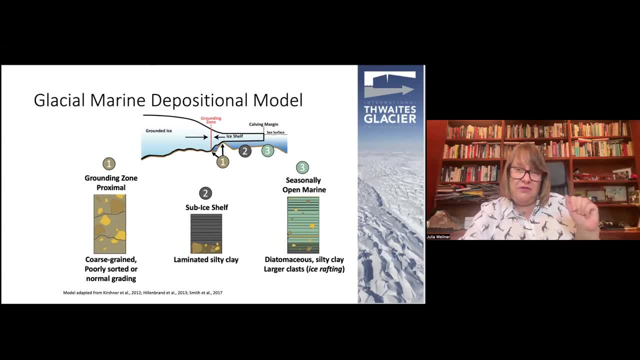 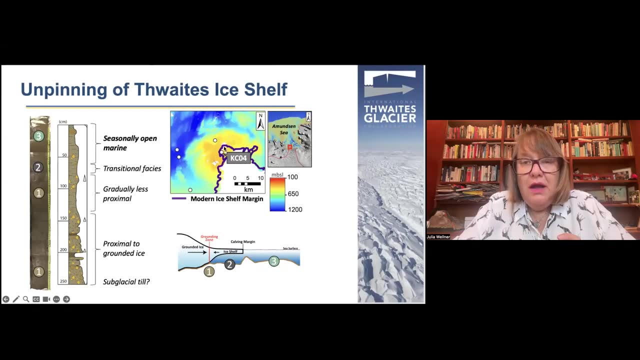 these different facies stack up one on top of the other, And so I can show you that here, um, where we take a core, uh, from this high area, or pinning point immediately adjacent to part of the Eastern part of Thwaites, Glacier, Um, and at the base of that core we have that. 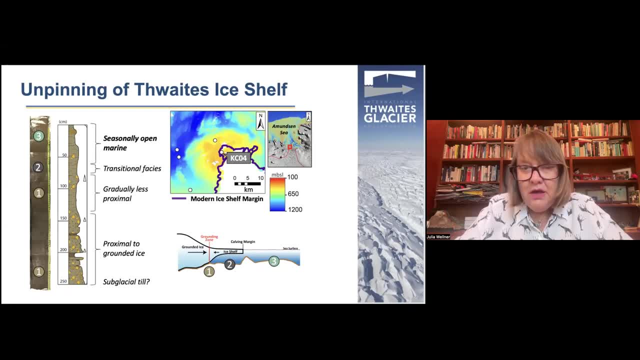 coarse, unsorted facies from zone one which is formed underneath ice or very close to it. Then, as we move up through this core, we get to the transition faces of laminated silty clays and a lower sedimentation rate, And then, at the top, 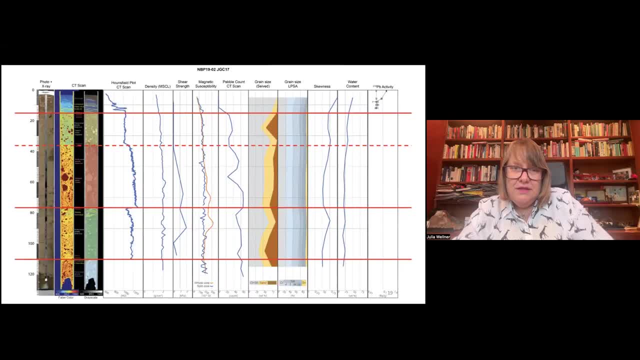 seasonally open marine. Uh, this is a figure um sort of highlighting all of the data um that we, as sedimentologists, collect in order to understand past records. I'm not going to talk through every type of data, but rather just highlight that we do a variety of measurements. 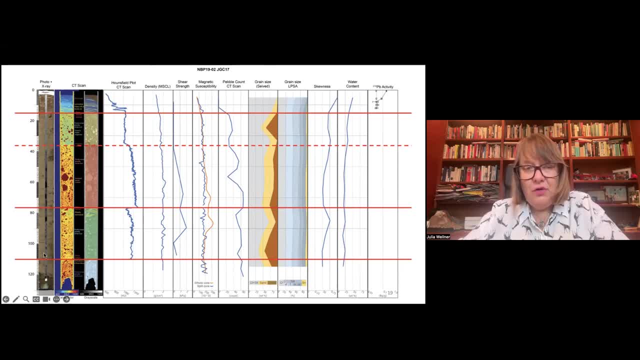 on the left is a photograph of the core with an x-ray strip laid over the top of it, And in the second column here is a CAT scan of the core. Uh, these are the same as medical CAT scans that you might receive yourself, but ours are done at a vet school where we are allowed. 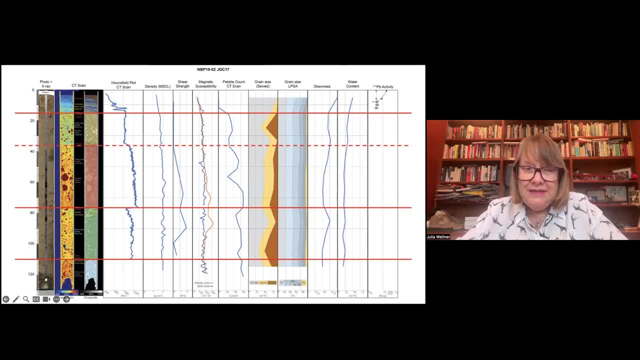 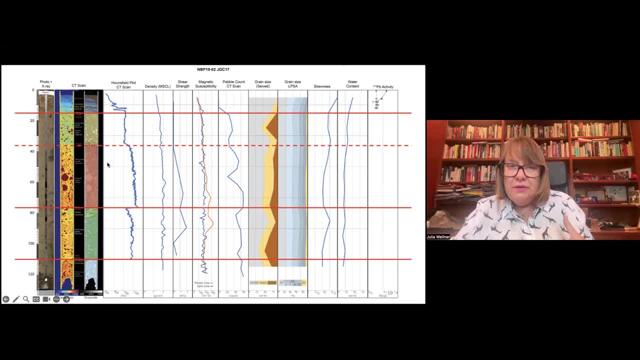 We stack that up with a variety of other measurements that we do on the core, including things like magnetics and individual particle sizes, And then, at the very far right, you see the ages that allow us to date the core. These are led to 10 ages that I showed you from my lab. 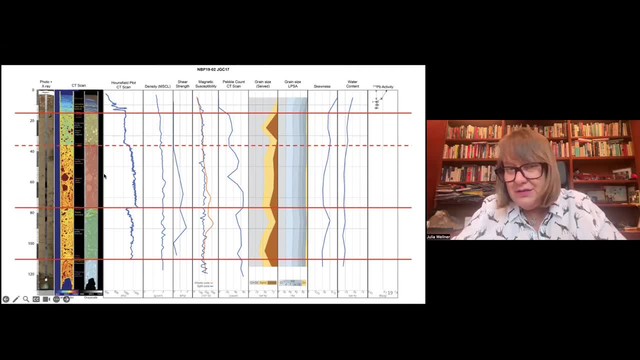 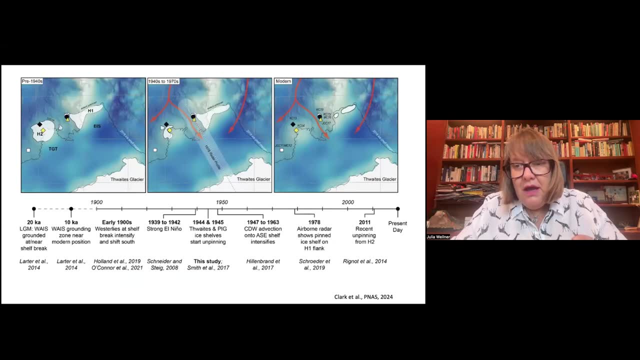 That only gets us back about 100 years, So all of this is older than that. but we're interested in that pre-satellite record, And so the paper that was published by my student, Rachel Clark, a week ago in PNAS this: 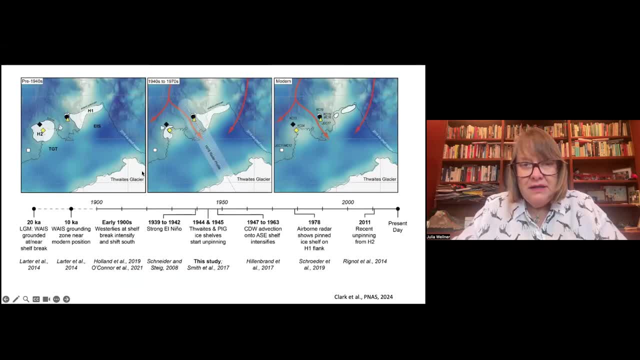 is the summary figure And to get you oriented, here is Thwaites Glacier in white on the bottom, And this is where we have ice floating. today is this masked area And out front, this is the Thwaites Glacier. Out farther is today's ocean. 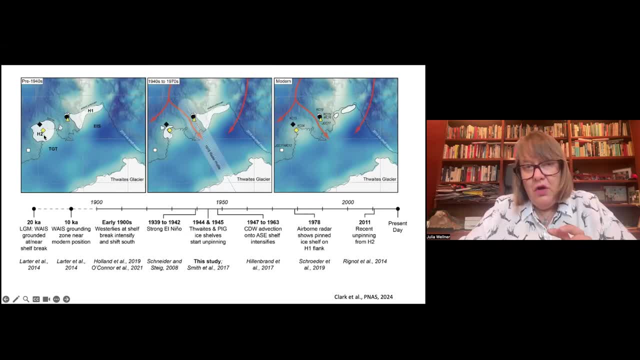 And in the cartoon in white is where we have interpreted ice to have been pinned pre-1940s. And again, that's based on a series of sediment cores, interpreting the sediments and the ages. And then we step through that over time and from the 1940s to 70s we're able to see this: 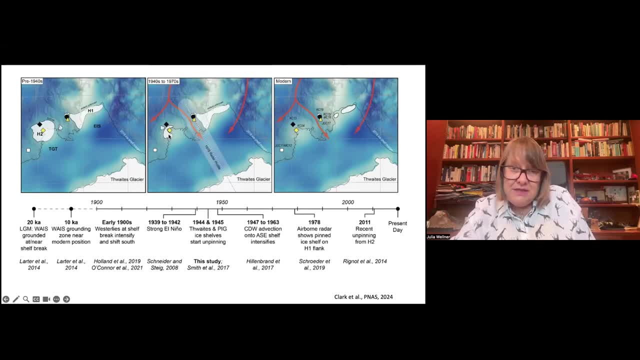 smaller area of pinning That's based on a combination of our sediment cores and a 1978 radar line that shows us where the ice was grounded, And then in the modern setting, we have grounded ice only in a few very limited places. 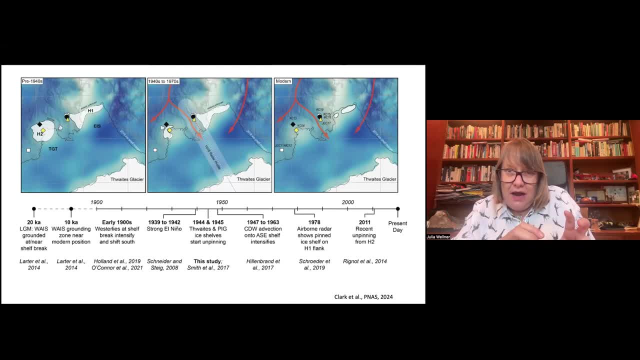 And that highlights to us how the ice has stepped back over time. Okay, That's not a huge amount of ice retreat from the 1940s to today, But it's at the same time as Pine Island Glacier, So we've dated Thwaites to be at the same time as Pine Island. 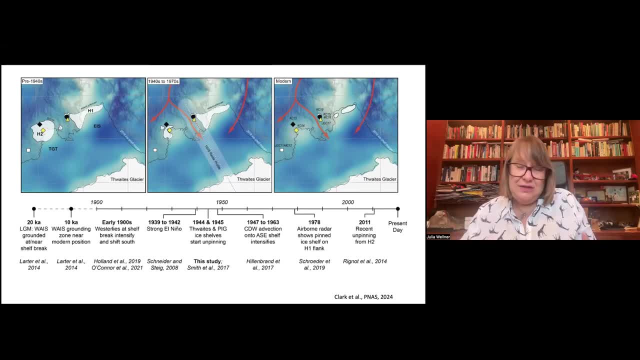 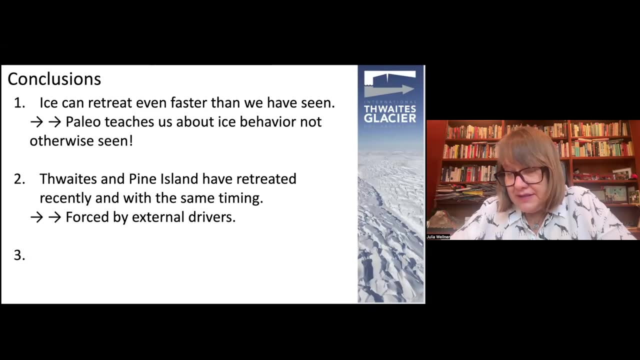 And what that shows us is that they are being forced externally, And so my second conclusion for you is that Thwaites and Pine Island have retreated recently, since the 1940s, with the same timing, And that shows us that they are forced by external drivers, quite possibly by the early 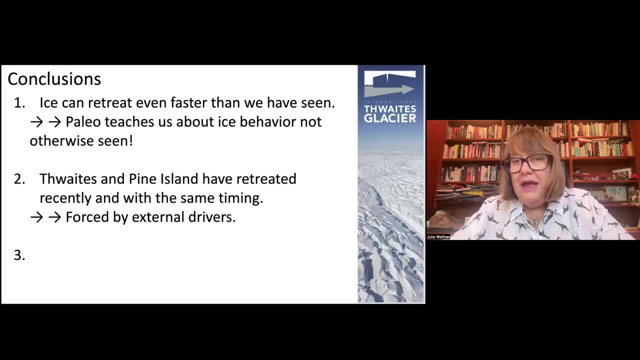 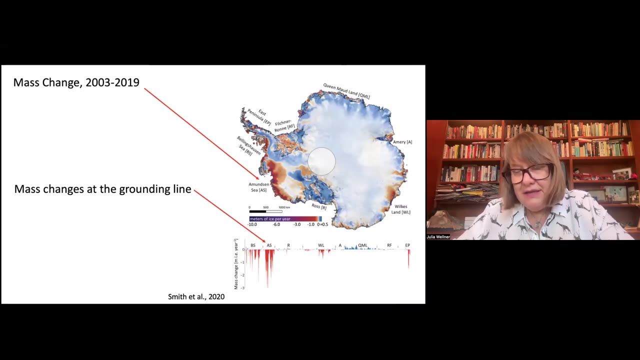 1940s El Nino, Because they are retreating in conjunction with each other, it is not likely to be just internal dynamics, And very quickly. as you know, Thwaites and Pine Island are continuing to retreat. This is now a different image. 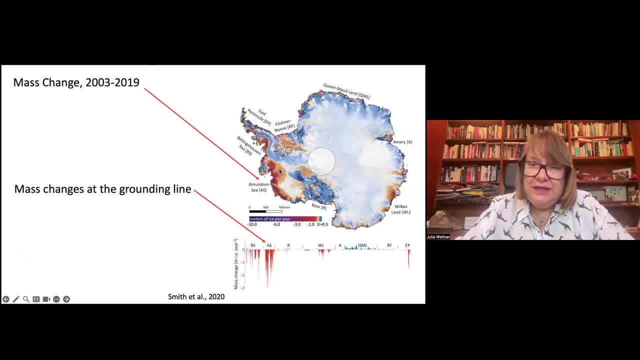 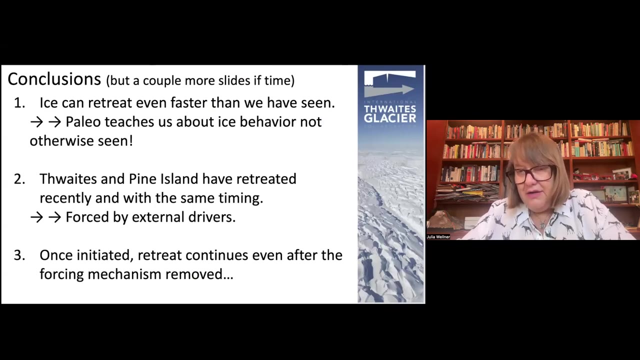 This is a mass change from 2003 to 2019.. And particularly at the grounding line, we can see how Amansansi stands out, And so the third conclusion for us is that, once initiated, retreat really continues even after the forcing mechanisms are removed. 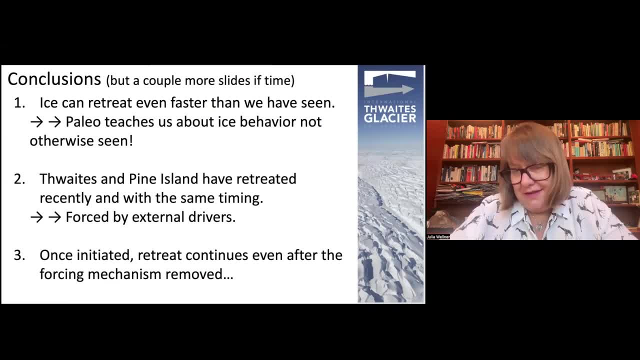 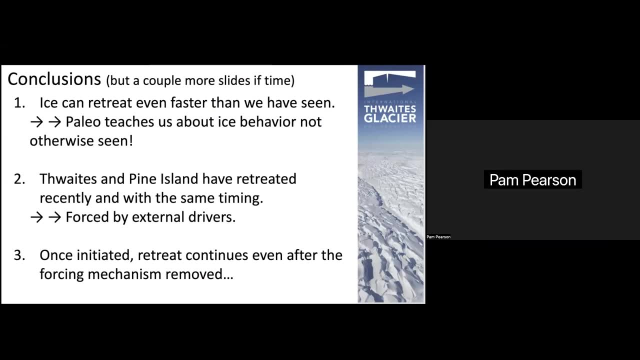 So I think I've hit my time limit and I'll just pause right there. I don't want to answer any questions. Thank you, That was really. it really really explained what is a very complex paper and what it's based on. 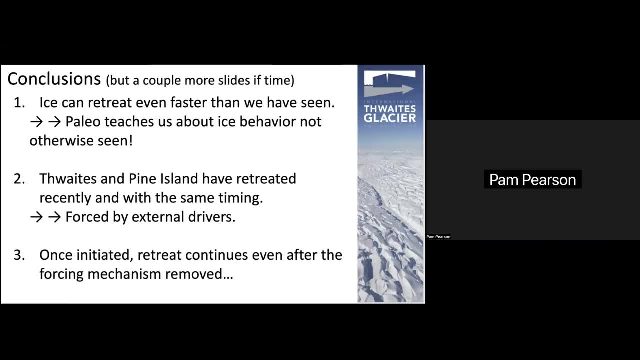 We have a few minutes for questions. We did start, Julia, so you're certainly welcome if you had anything more in your presentation you wanted to give. That's fine, But are there any questions? And if not, I'll ask- and this is actually sort of related to the next presentation as 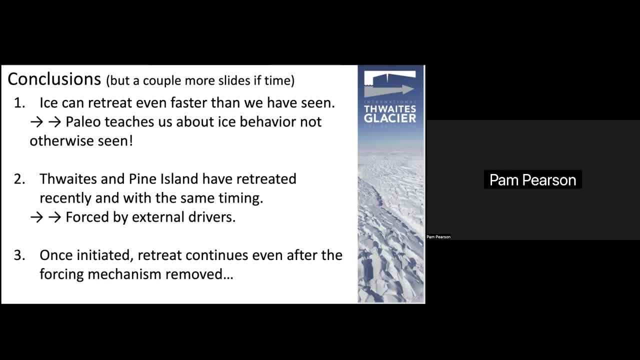 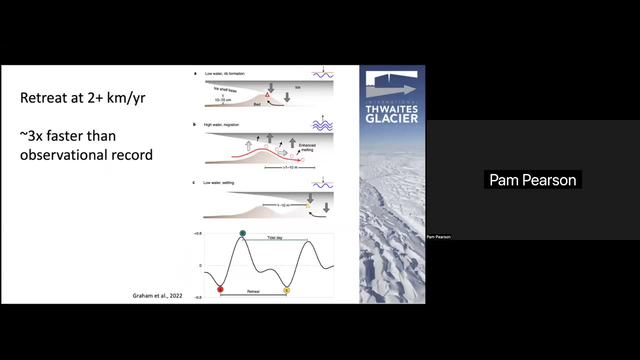 well, When does an ice sheet become an ice shelf? In other words, we're talking about grounded ice shelves in the next presentation. If something is grounded, does that make it part of the ice sheet, which maybe? there's no firm, fast answer to that. 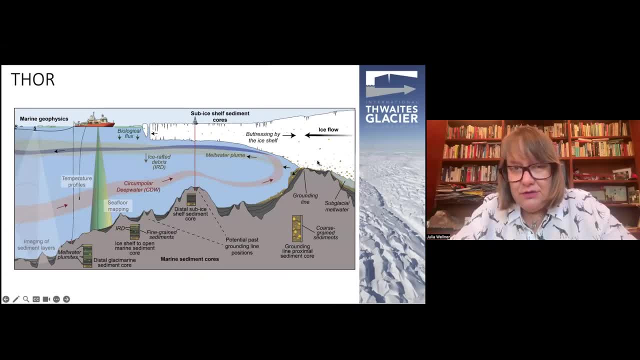 No, there is a very clear answer. So, going back to this cartoon showing how we set up our project to begin with, the ice sheet is the material that is back here and is behind the grounding line or upstream of the grounding line, all of the ice that is still directly interacting with the sea floor. 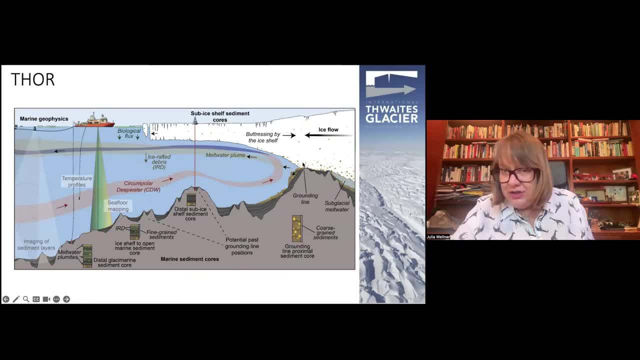 or the bedrock on land. That is the ice sheet. And the floating ice shelf is the material that is already buoyant in the water column And the position between them where we go from ice that is resting on the sea floor to ice that is loading in the ocean. that contact point is called the grounding line. 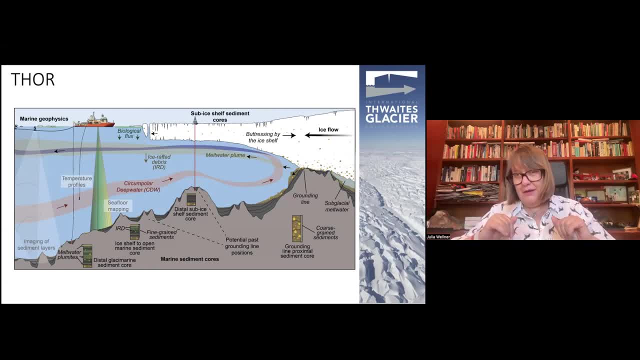 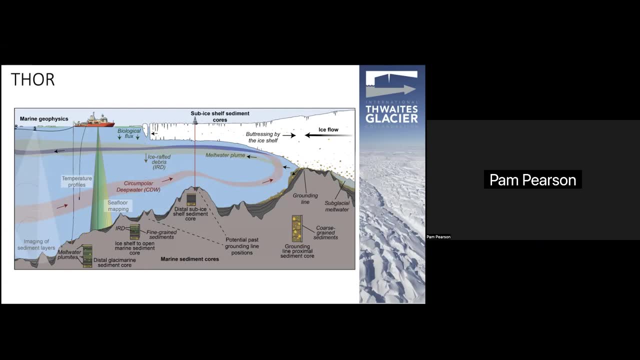 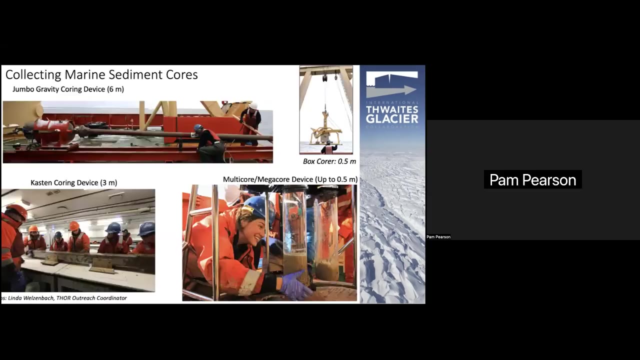 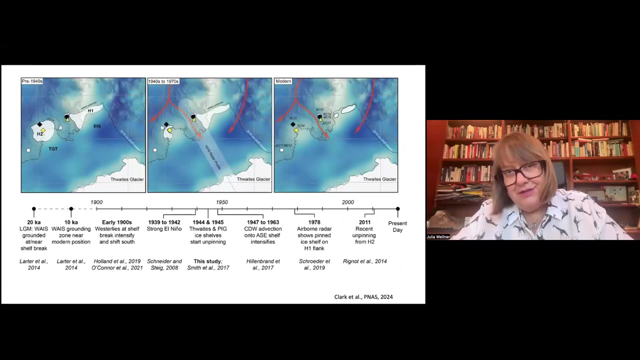 It's not really a line, It's a zone. Yeah Right, But if an ice shelf is pinned, that means it's all grounded, correct? Yes, That's my question, That's my conclusion. Sorry, Yeah, Sorry, if I well. that's, yeah, that's a good question. 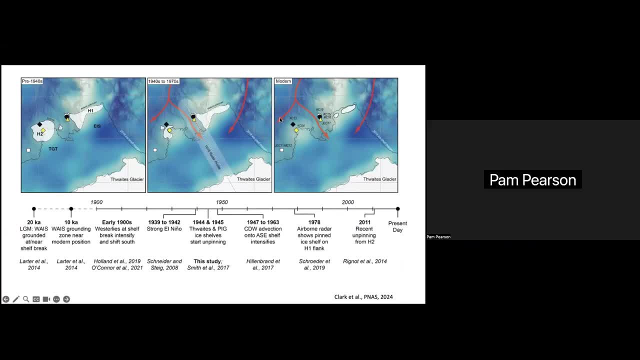 I think now we're in semantics, you know. So here in today. you know we call this whole area out here the eastern ice shelf, Correct, You can see an outline here in the bathymetry. Yeah, And it is pinned today just out here. 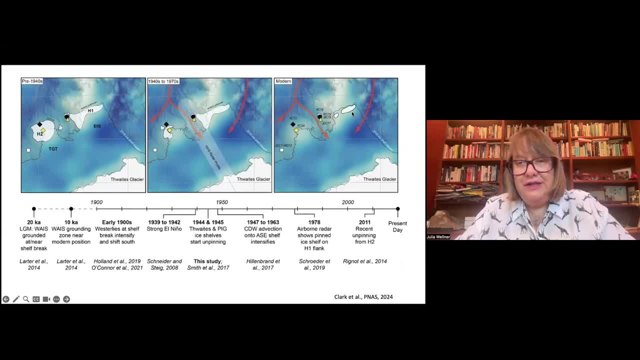 I would say we would still call that ice shelf. It's just ice shelf that's resting a little bit. This is the significant grounding line back at the bottom of the diagram And this little bit of floating ice is just. it might be pinned there, but it's just resting. 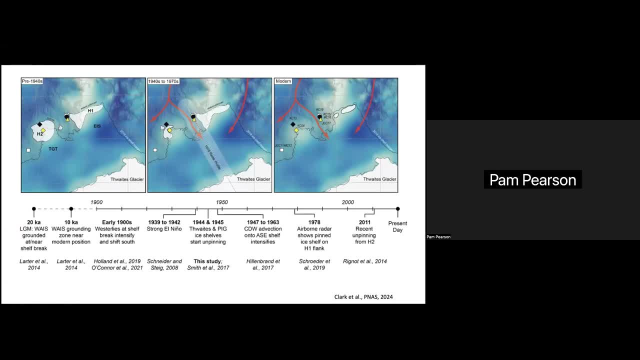 It's not a true grounding line, Exactly Okay. Okay, All right. So we have a question here from Matt, from Perrin Pletnikoff, I believe, from the Wilson Center: How did two glaciers simultaneous retreat, show external forcing? Well, that's a good question. 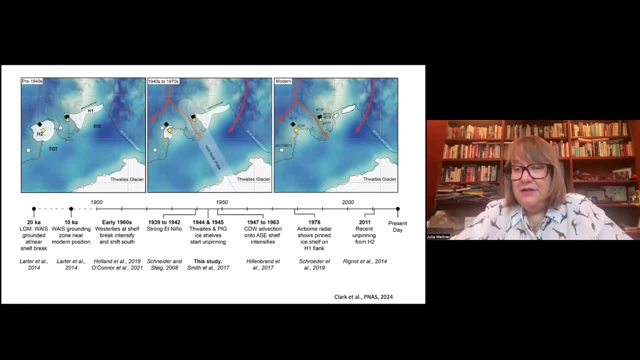 And I tried to carefully address it, to say that it doesn't prove it, It just suggests it. And the reason is just like if you look at I don't know, a bunch of trees that fall down, One tree might fall down. 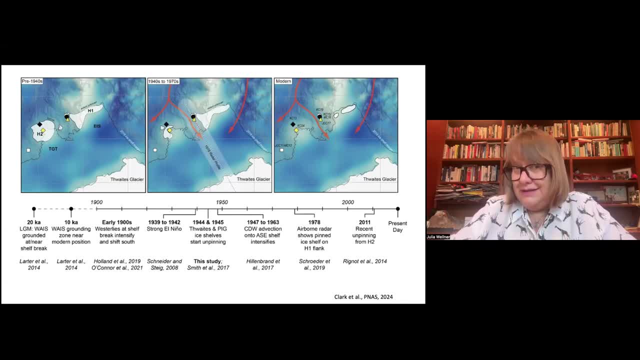 Yeah, Because it's old and it dies and it's sick. But if a whole bunch of trees fall down tomorrow, it's far more likely that a windstorm pushed them down, And so we look at these glaciers in the same general context that any one glacier might. 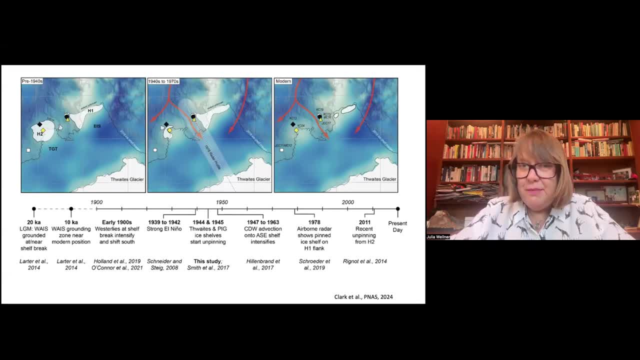 be behaving in its own way, And some of the best examples for that, Okay, Are when we go back into the paleo record, we have a lot more data from glaciers on the Antarctic Peninsula. We've worked in the fjords there over many years. 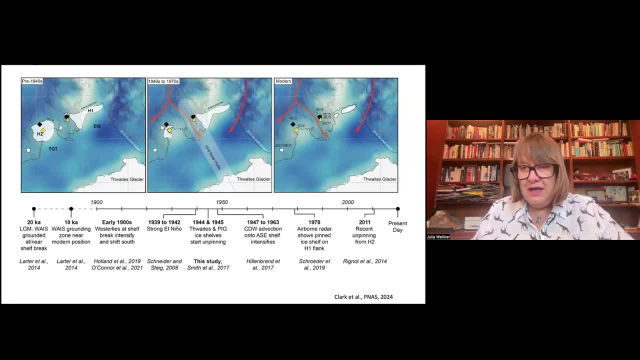 It's easier to work there than it is at Thwaites, And there, when we go into the paleo record, we see one glacier advances at 8,000 while one retreats at 8,000.. And then at 7,000, they might shift. 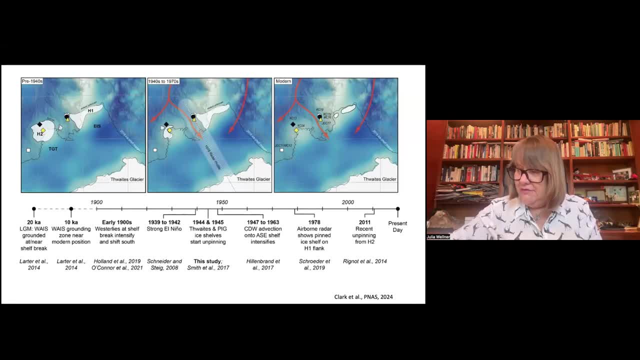 And all of that is related to each glacier. And so we look at these glaciers, even though they're nearby, each other sort of changing based on their own pinning points, their own random calving cycles. But today in the peninsula, meaning over the last few decades, we see broad scale retreat. 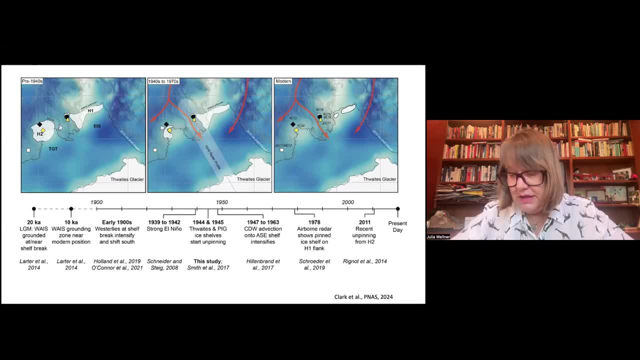 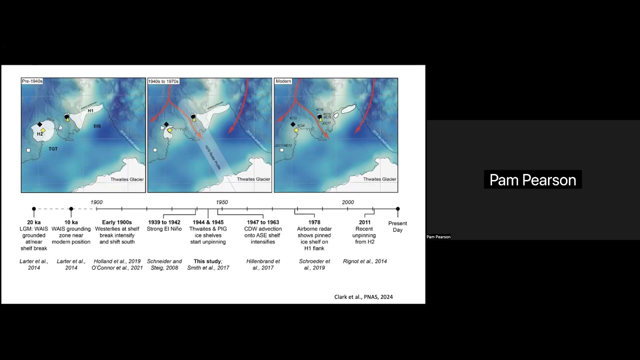 of most of the glaciers- not all, but most- And that suggests that those are responsible, That those are responding to atmospheric temperatures warming there. So it's not proof, but it is very strong suggestions of correlation. Thank you, Yeah, And could you? we'll go ahead onto you, Birdie next. 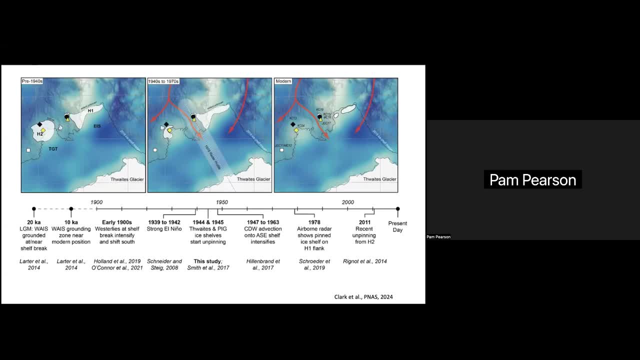 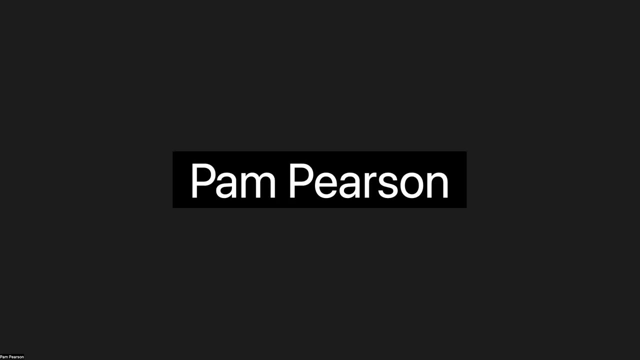 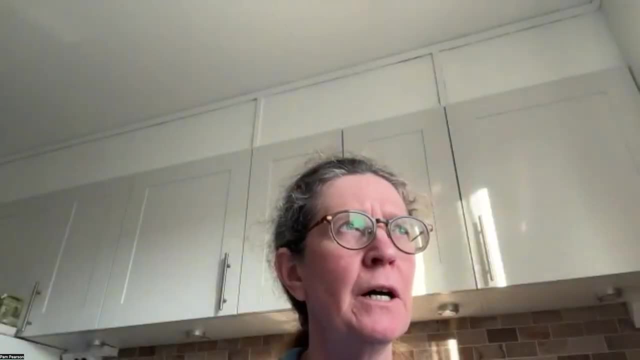 So if you want to start getting your slides up- and Julia can stay until the end and so we can have a broader discussion- then as well. But do you actually have almost a year on you? Yeah, I do have a year tracking, And the reason I'm asking that is that we know in Greenland, for example, there were 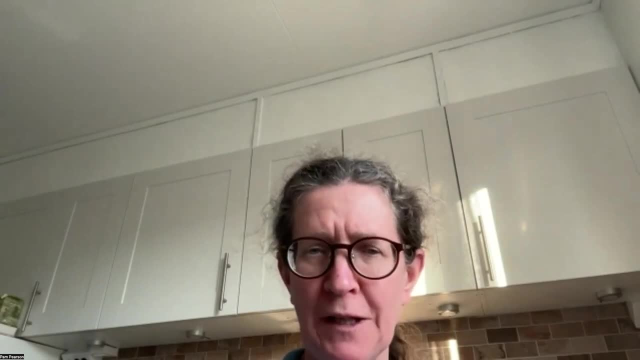 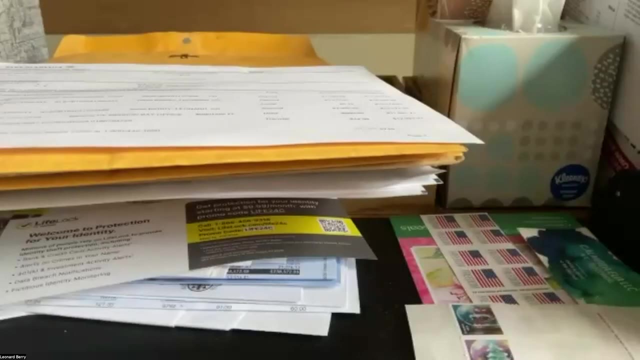 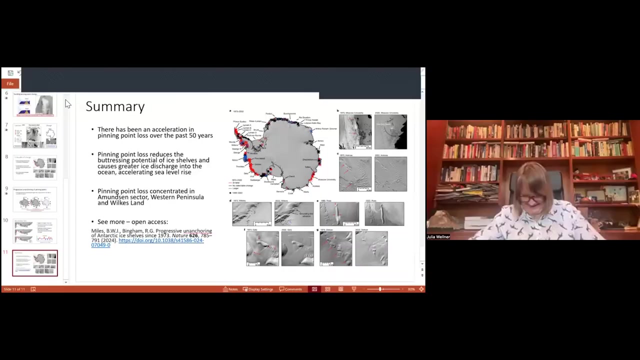 signs of World War II and a decline actually in industrial activity because you had black carbon actually going down during that period. Can you actually give a you know, 1940, 1939 to 1950? Is it that exact? Yeah, that's a great question. 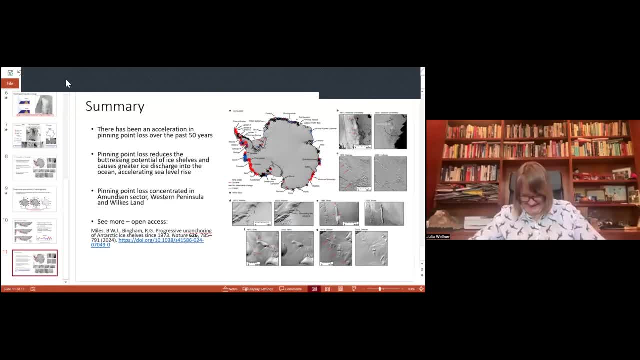 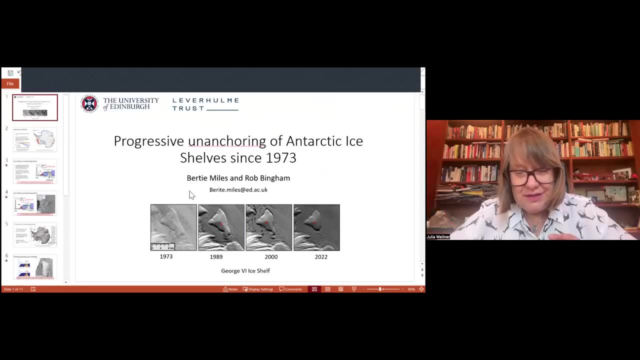 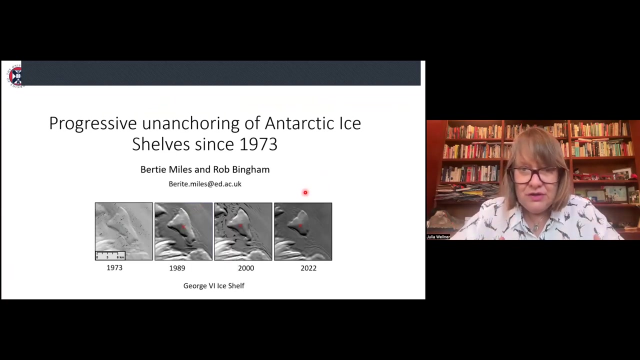 A really great question to think about. The answer is broadly no. Okay, So we do not have specific details like that. One, our age models are more plus or minus a couple of years, and that's the best you can do. But two, there's no evidence of direct fallout or ash or soot of any type. 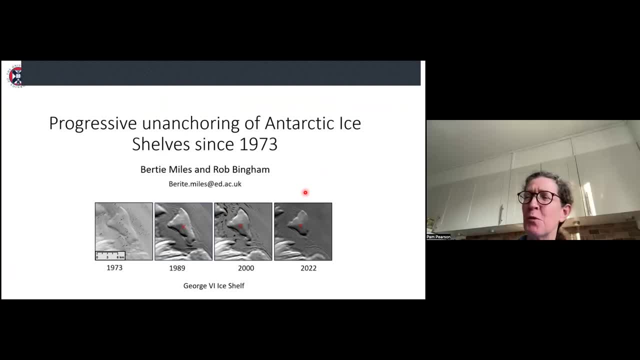 Oh no, Yeah, There wouldn't be in Antarctica. Yeah, But I'm thinking just more in terms of, yeah, warming. What was going on in the area? Yeah, What was going on in the 40s? Yeah. 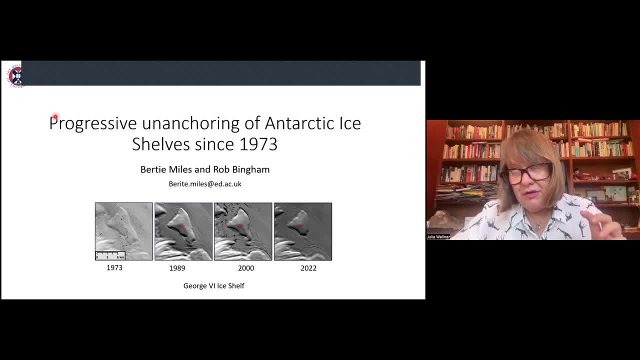 No, we don't, We do. I showed you that I measure lead 210 as well as cesium. Cesium 137 is a bomb product, Yeah, And so I do use that as part of our dating, but the only thing we're able to date is the. 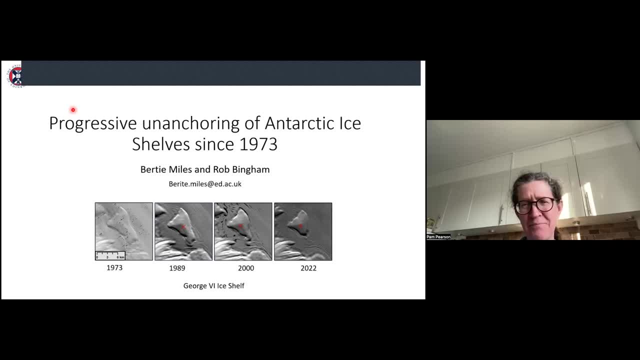 nuclear test ban treaty Right That far south. Yeah, Okay, Thank you. So now again staying in Antarctica, but looking at ice shelves, Bertie, please go ahead. Yeah, Hello everyone. So yeah, I'm going to be talking about a recent study on the progressive unanchoring. 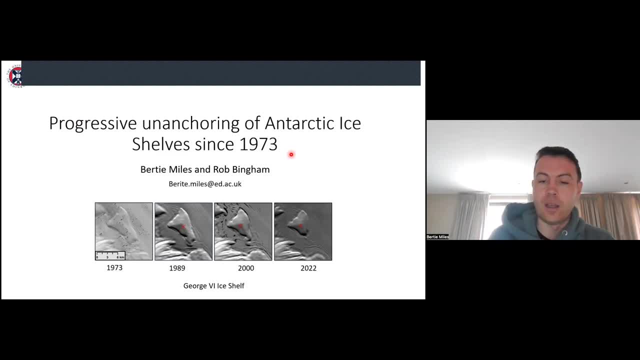 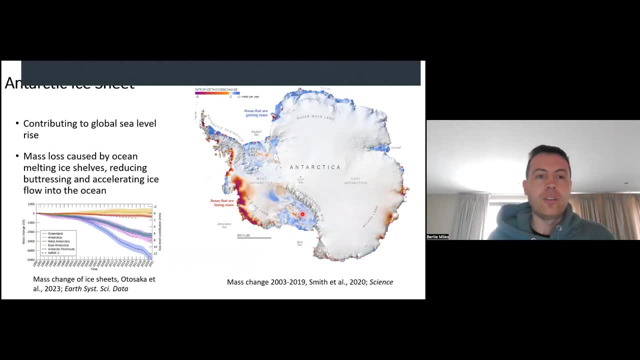 of Antarctic ice shelves going back to 1973.. So yeah, Another quick, brief background on Antarctica. As Julius talk said, it is contributing to global sea level rise. So this kind of figure in the bottom left is showing the mass change of the Earth's. 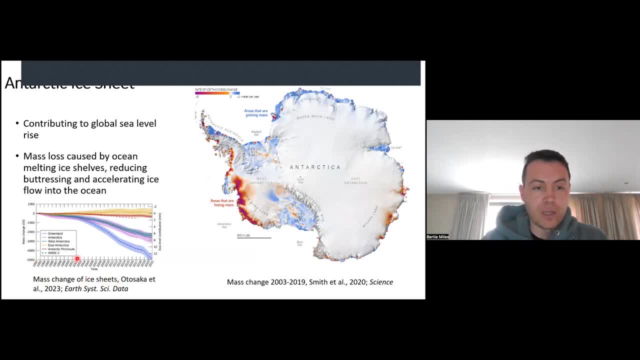 ice sheets going back to 1992.. And this purple line is Antarctica. You follow all the way along. you can see it's contributed about eight millimeters to global sea level rise since the 1990s. You can also kind of see this kind of acceleration trend. 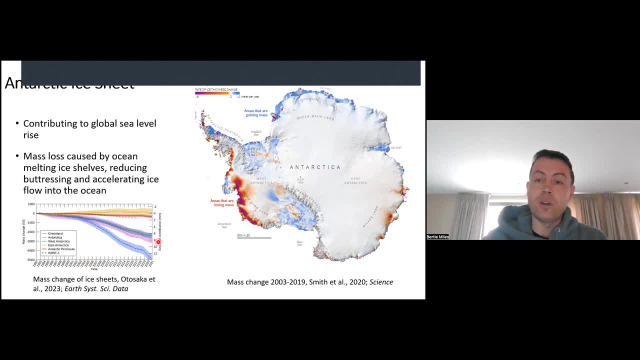 And if you look at the spatial pattern of that, so this is again the figure that was shown in Julius talk. Yeah, So this is the mass change between 2003 and 2019.. So it's formed, measured by a satellite, altimetry, a satellite called ISAT. 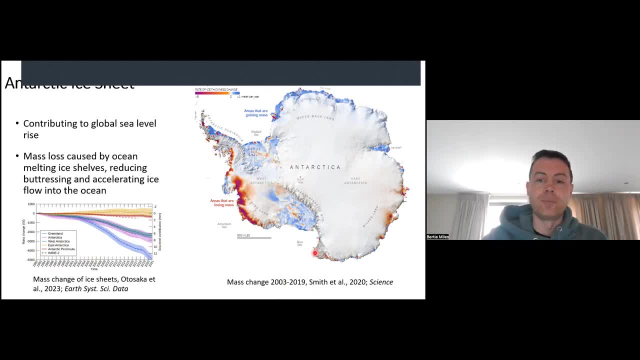 So it's potentially measuring the thickness change of the ice sheet And again you can see this kind of red where you're getting mass loss concentrated in West Antarctica. Again you can see sort of pine islands here and all along this kind of Western coastline. 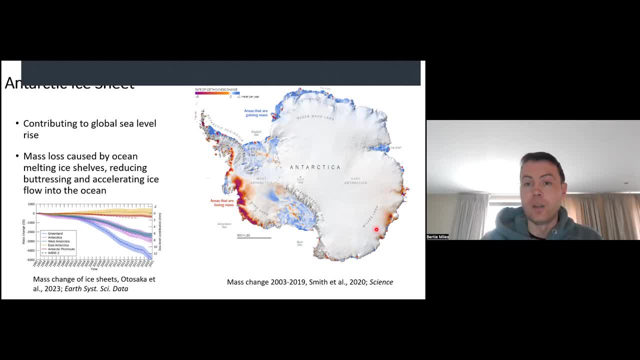 as well, And also in this area called Wilkes Land in East Antarctica. But very little change in this Queen Maud land region And the reason this is happening is, again, it's not because of this surface melt You might see in maybe Greenland or Svalbard or a mountain glacier. 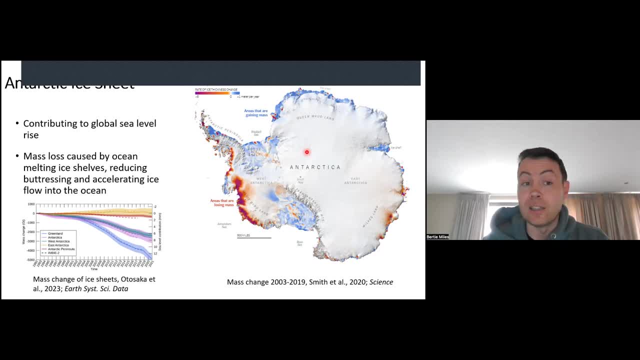 This is the warm ocean currents melting the underside of ice shelves, reducing the botching and accelerating ice flow into the ocean. So in this figure, the boundary between the grounded ice, the ice sheet and the ice shelves. it's this kind of thin black line. 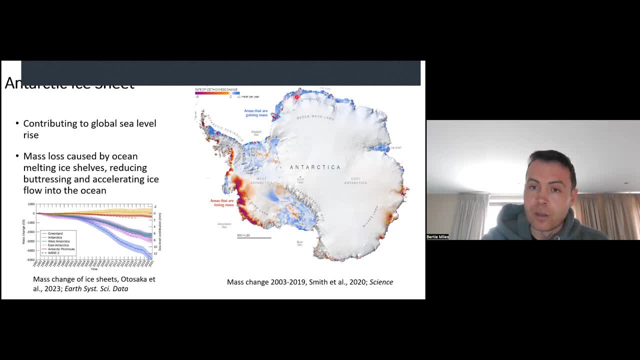 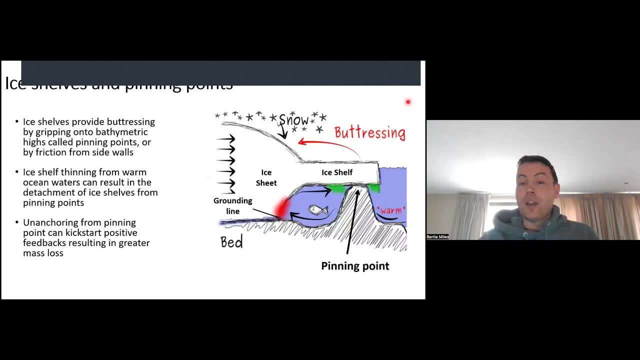 You can kind of trace it all the way around. So a bit more on to ice shelves. So you have an ice sheet, it flows towards the ocean, It begins to float at the grounding line and you get this ice shelf And the way these ice shelves provide the botchers thing back to the grounded ice is. 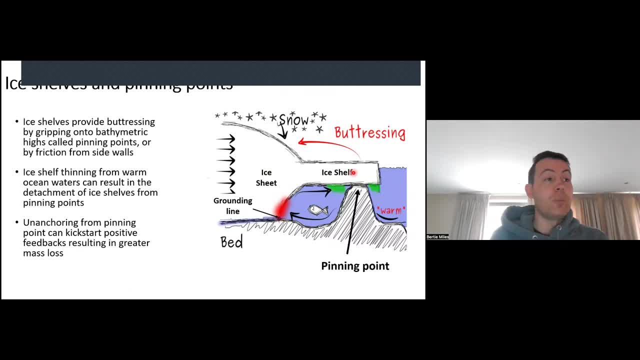 typically these things called pinning points. So these are topographic highs on the sea floor And you get an ice shelf flowing. They can be maybe five, 600 meters thick. They kind of run aground and anchor onto these pinning points. 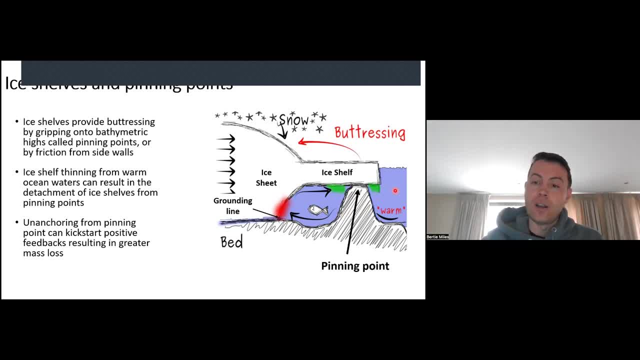 And if you can imagine warm ocean currents melting the underside of this ice shelf, you can imagine it would eventually thin and detach from this pinning point. So it's kind of like a ship unanchoring its anchor. You take that friction and buttressing away, then ice is going to flow much quicker in. 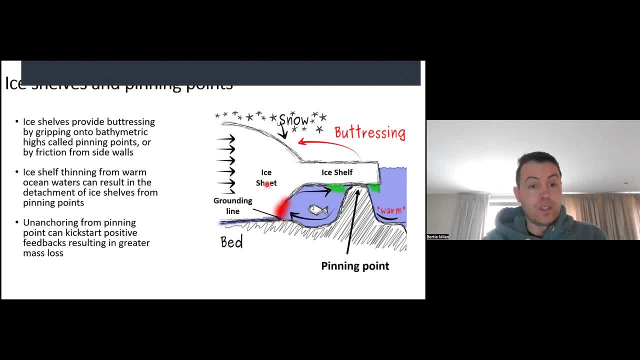 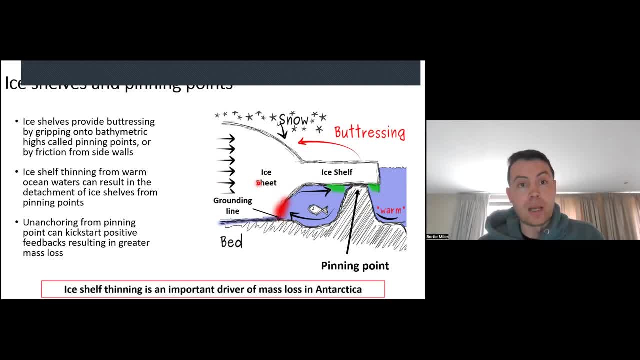 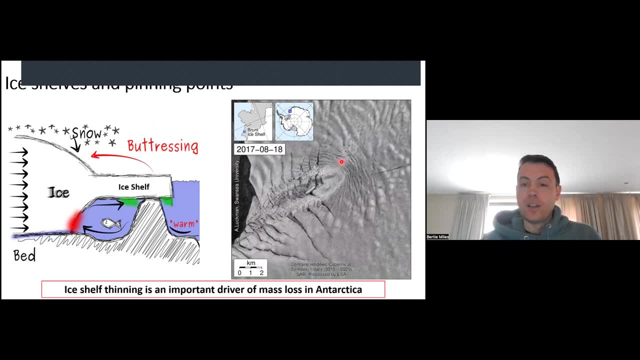 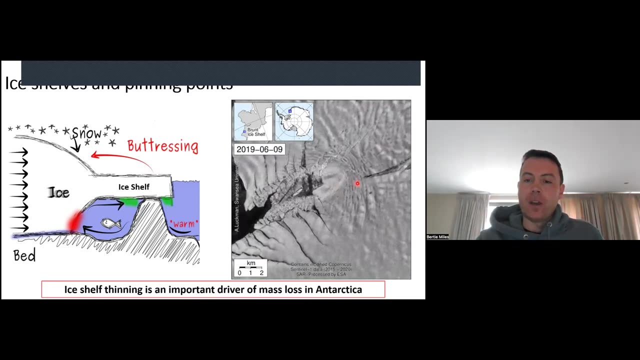 So really it's ice shelf thinning which is really an important driver of mass loss in Antarctica, And if you want to see an example of this pinning point, you can sorry someone's at the door. This is a series of radar images made by Adrian Lockman at Swansea University. 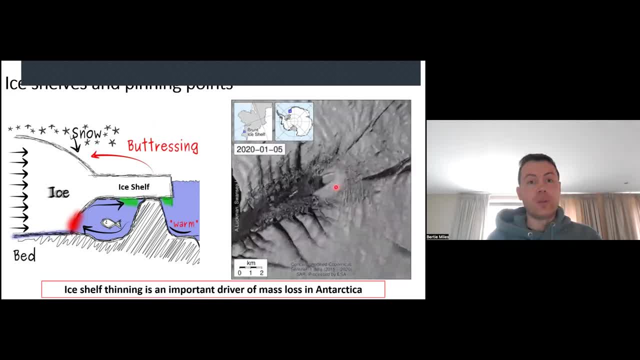 And what it's showing is that this is a series of radar images made by Adrian Lockman at Swansea University, And what it's showing is that this is a series of radar images made by Adrian Lockman at Swansea University, And what it's showing is that this is a series of radar images made by Adrian Lockman at Swansea. 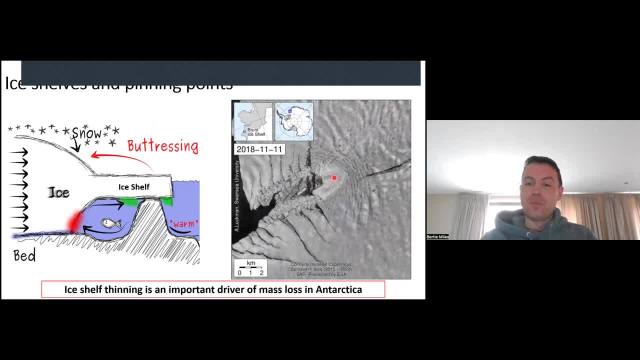 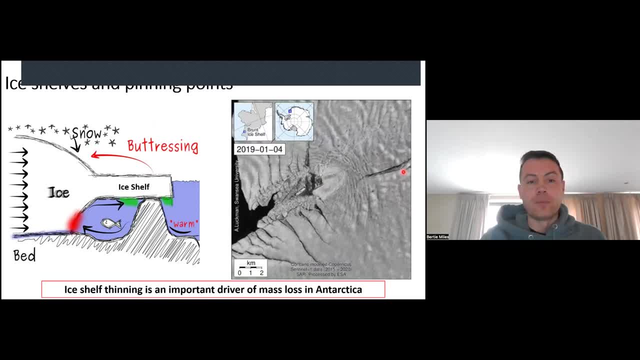 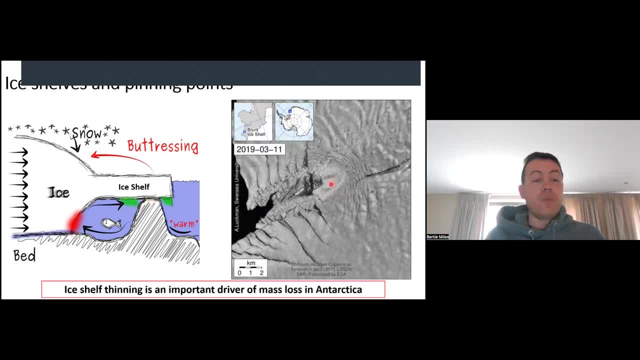 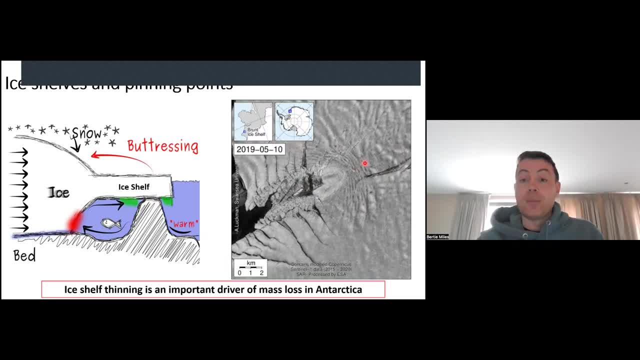 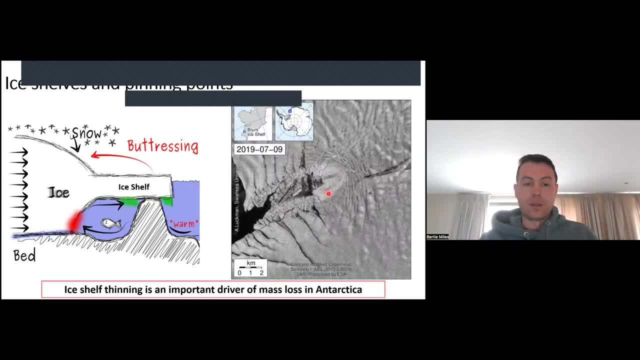 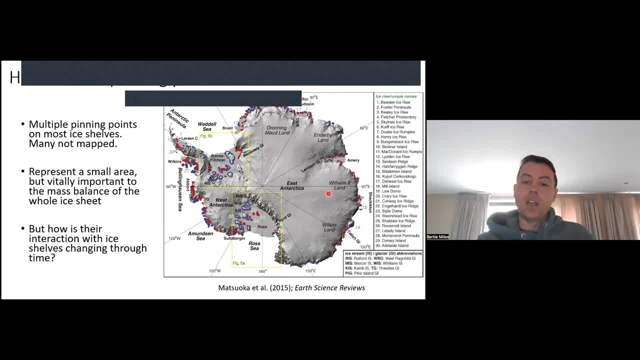 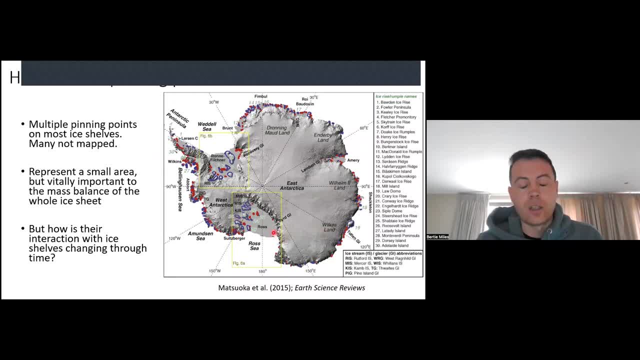 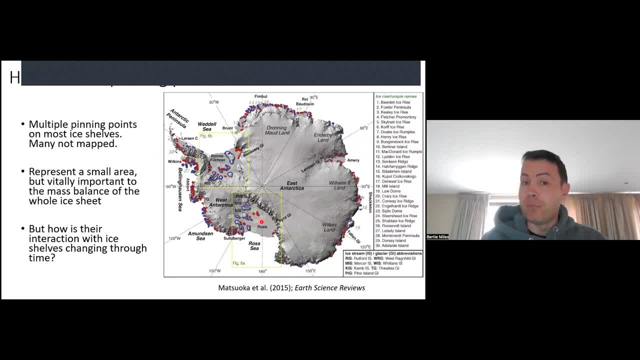 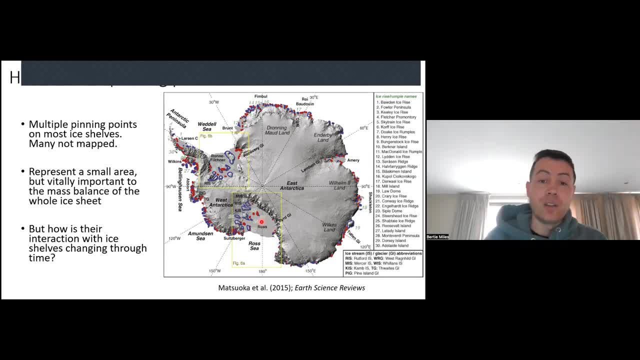 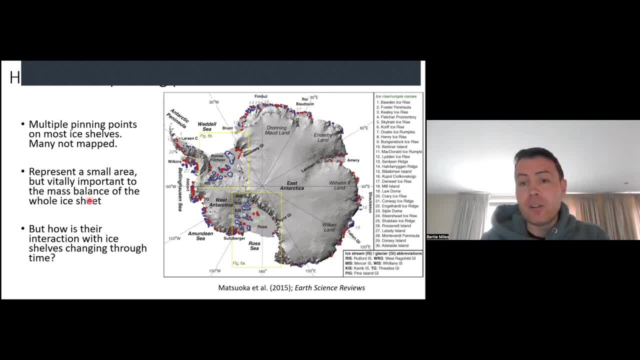 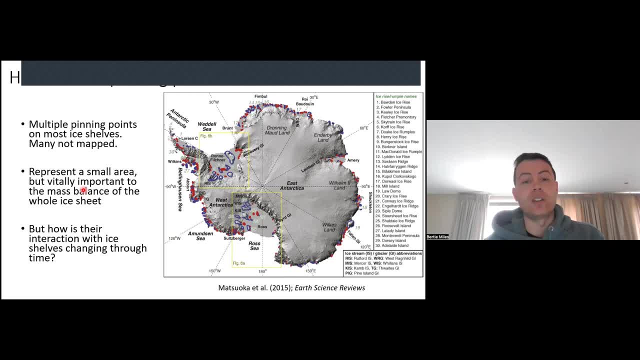 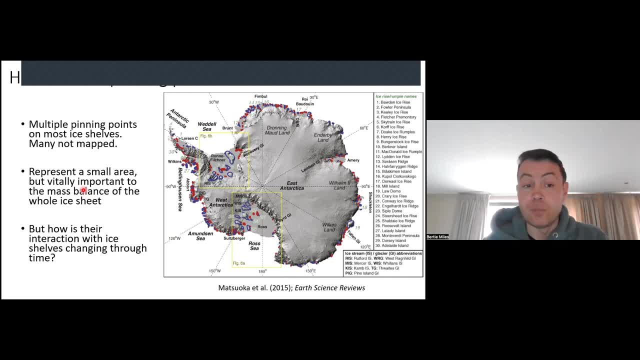 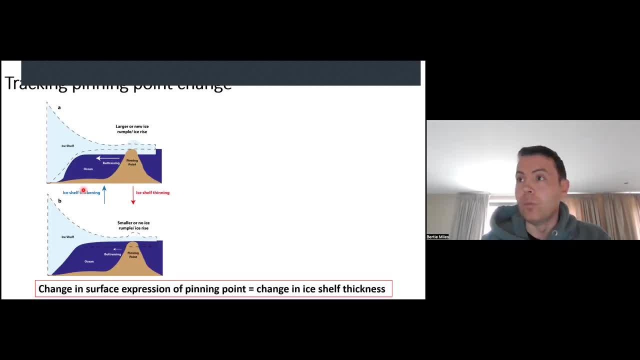 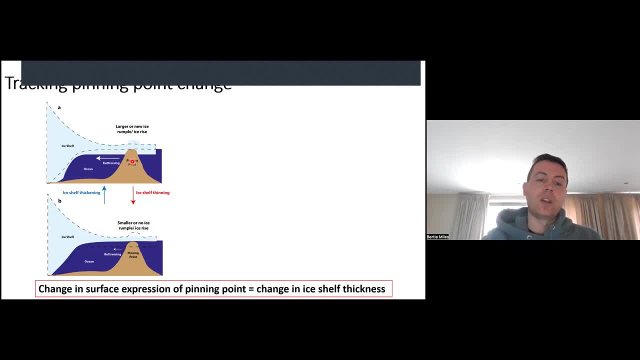 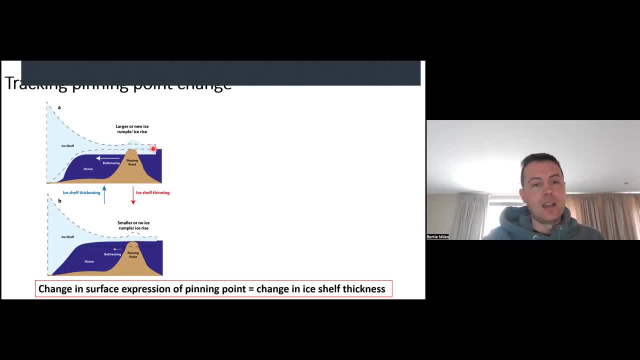 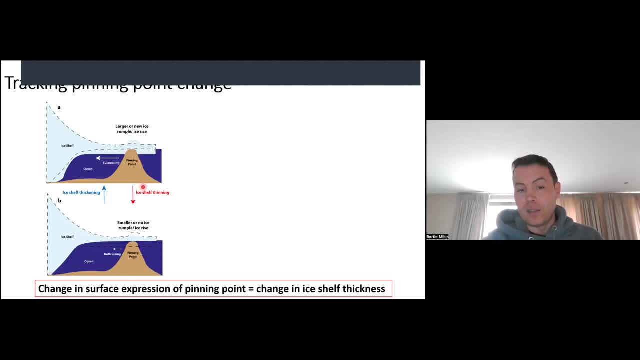 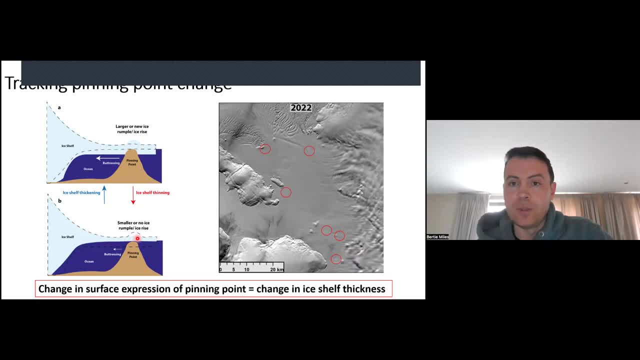 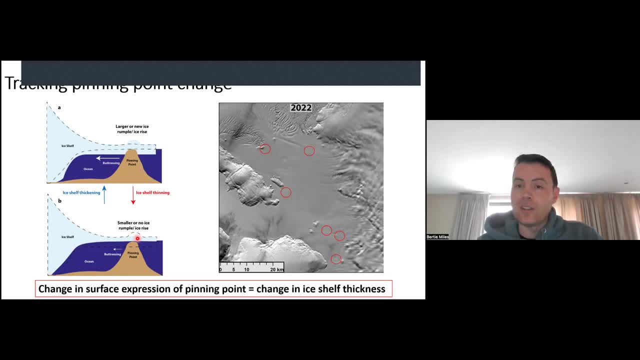 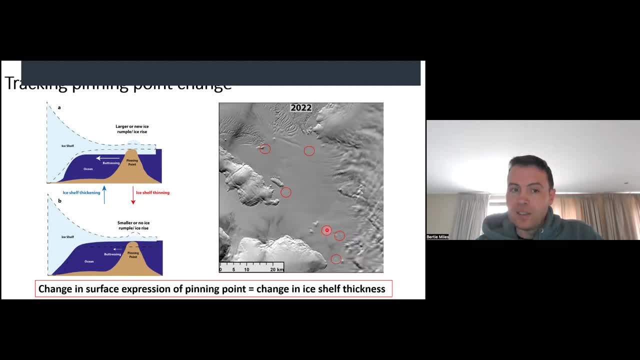 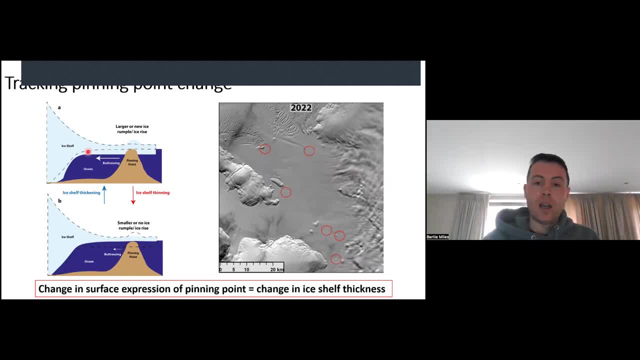 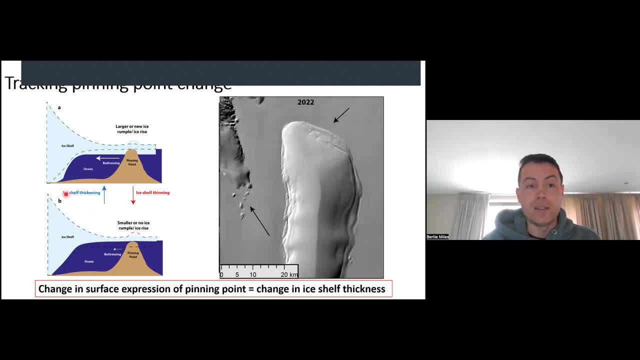 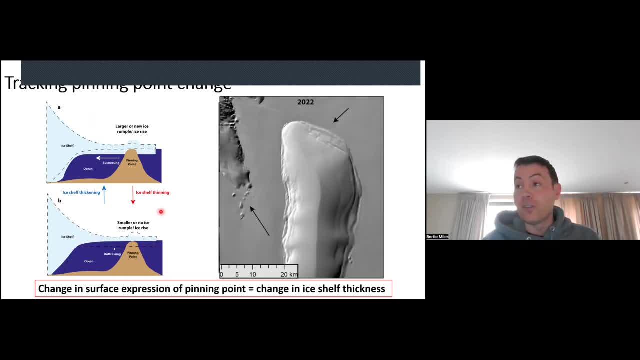 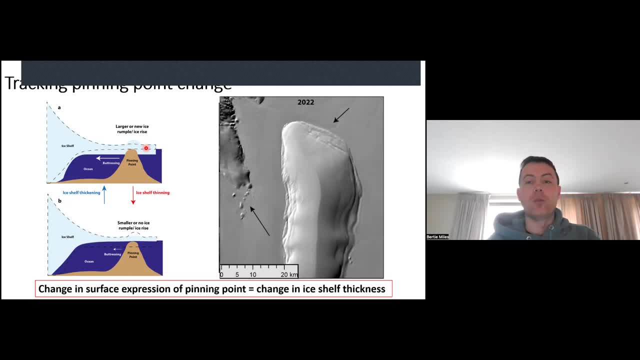 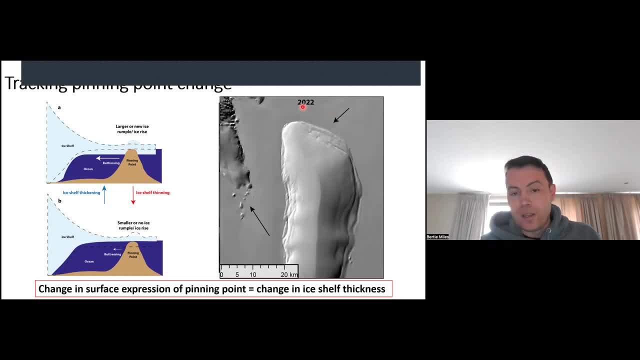 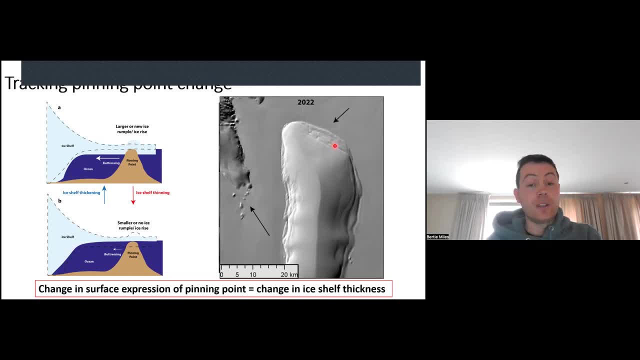 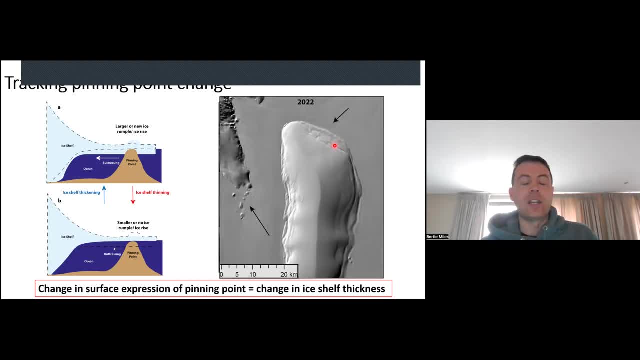 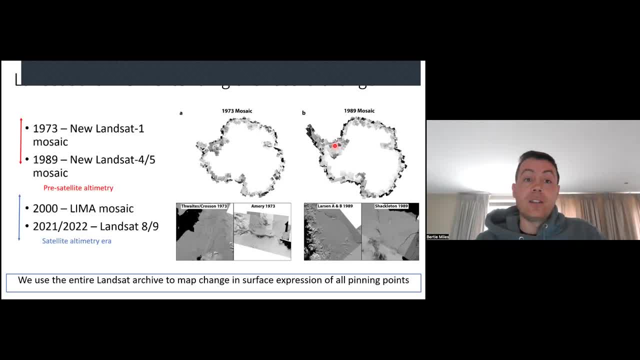 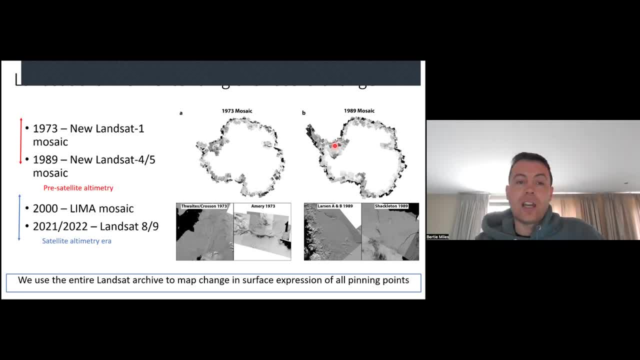 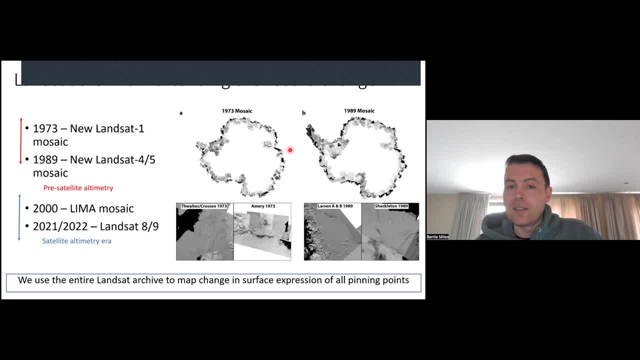 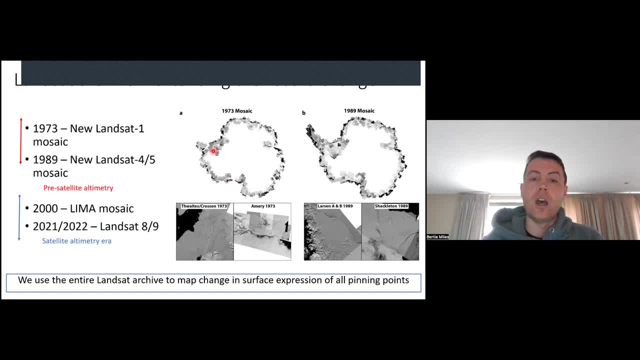 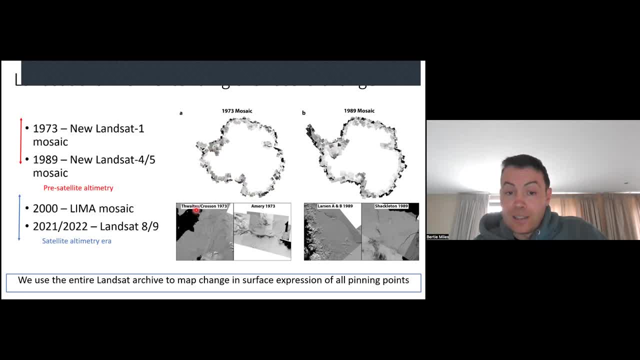 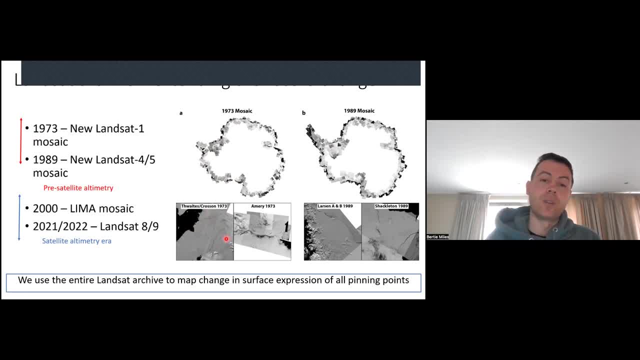 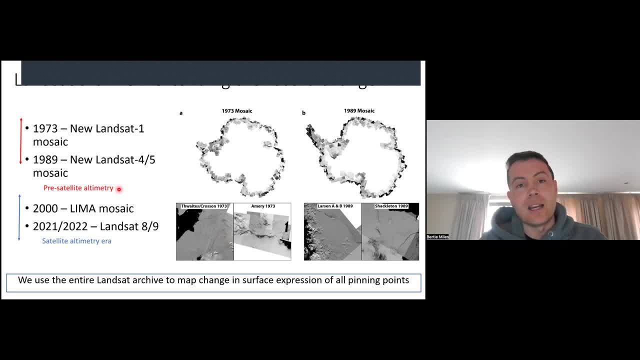 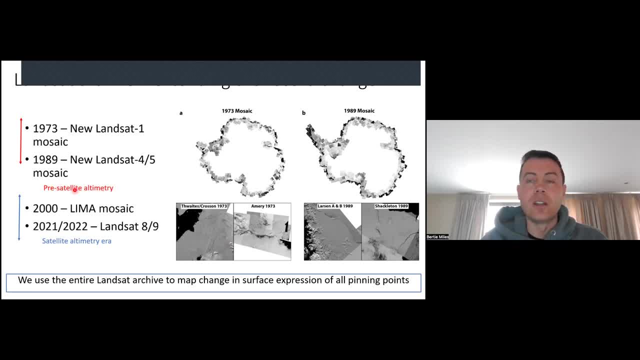 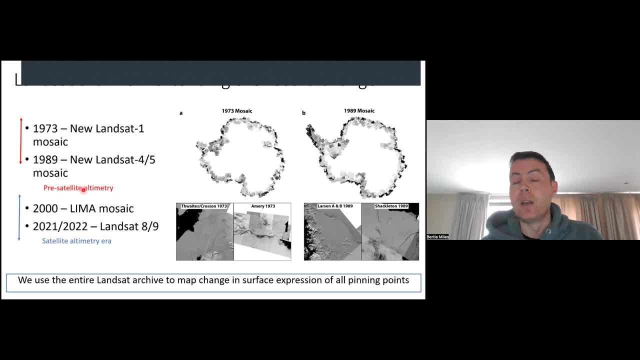 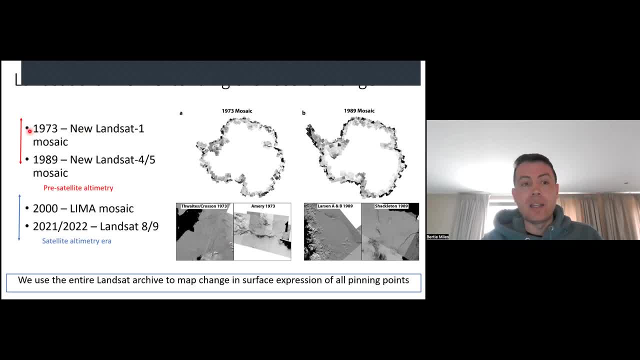 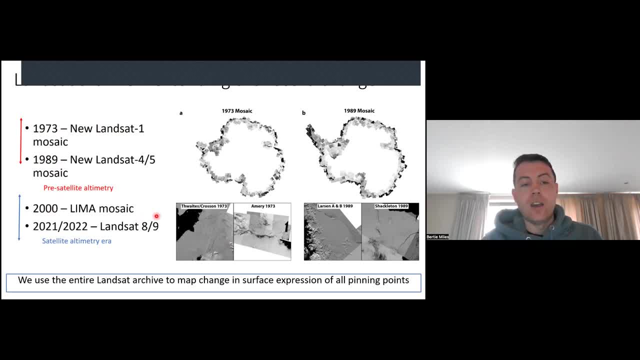 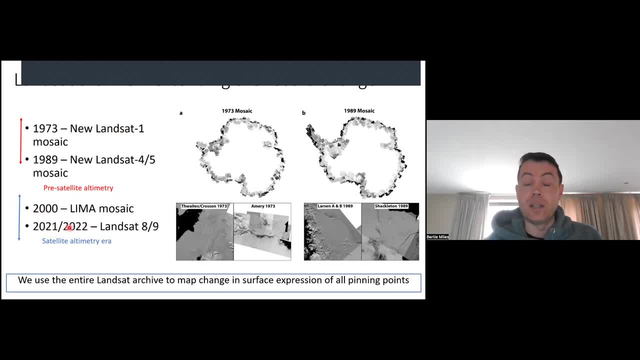 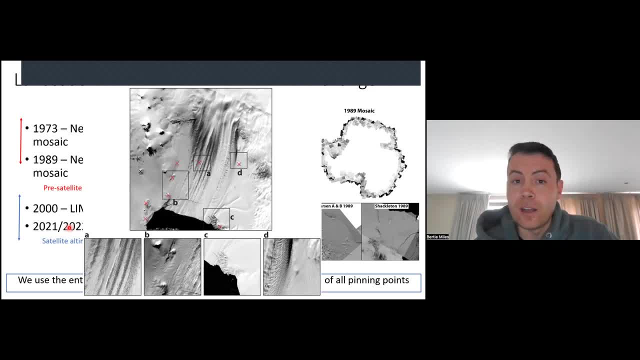 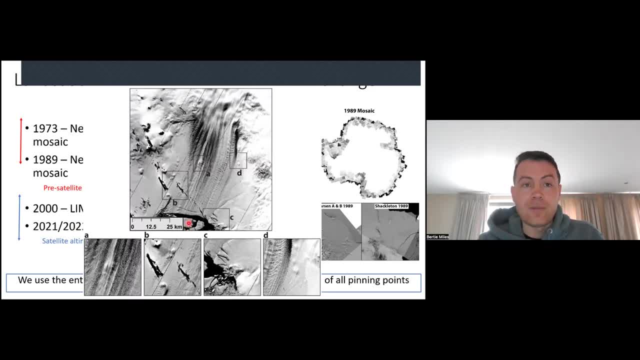 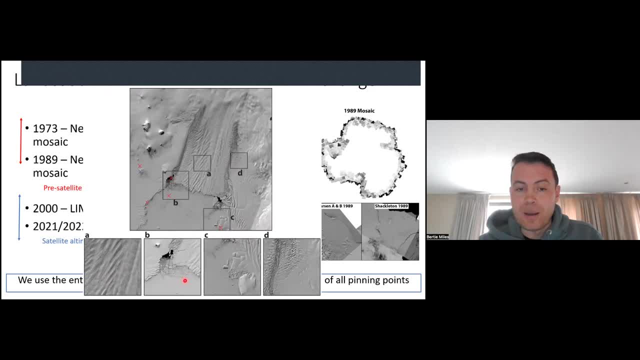 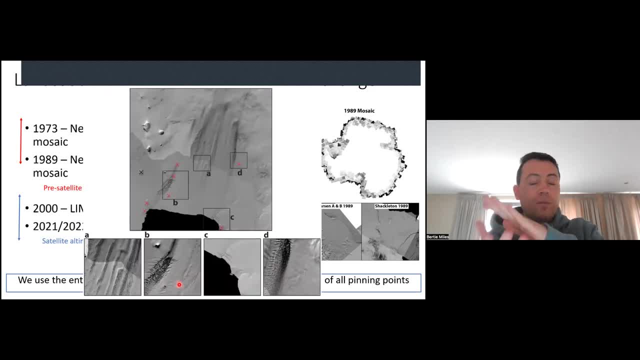 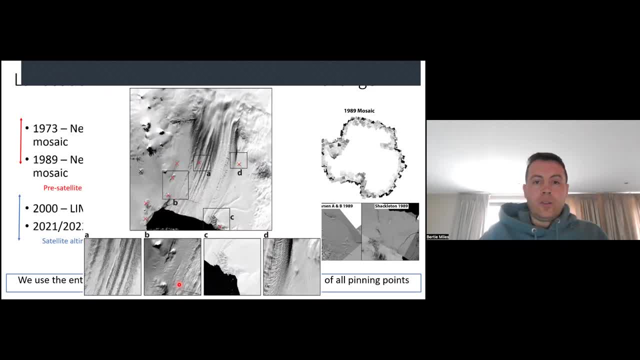 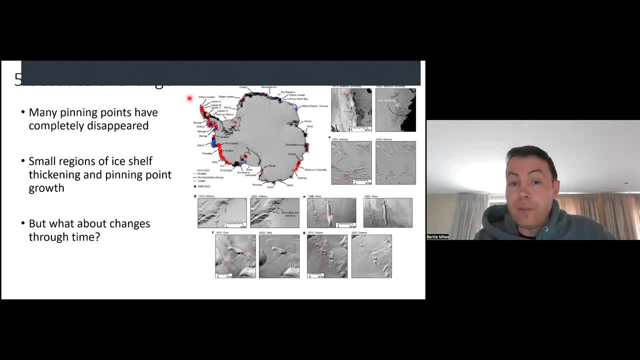 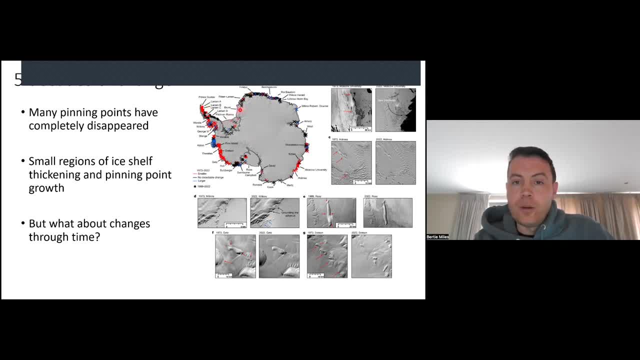 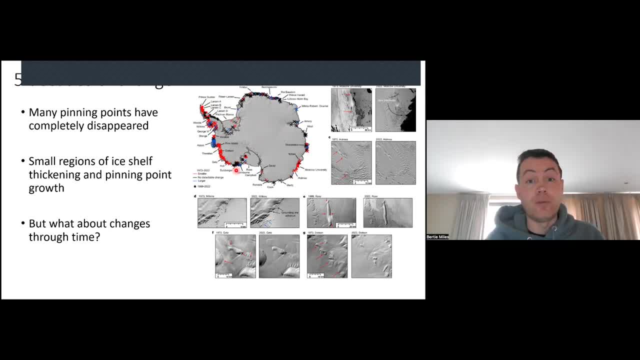 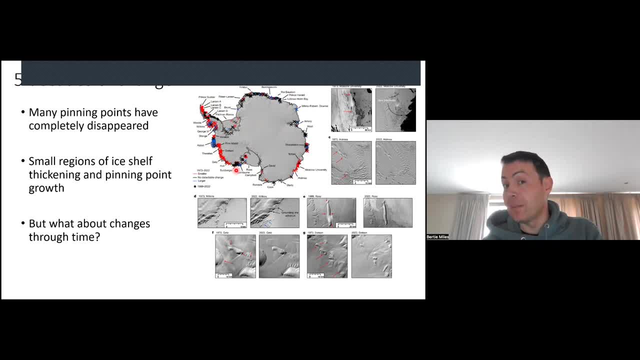 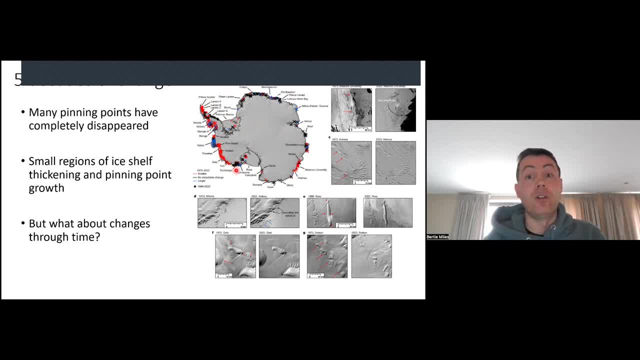 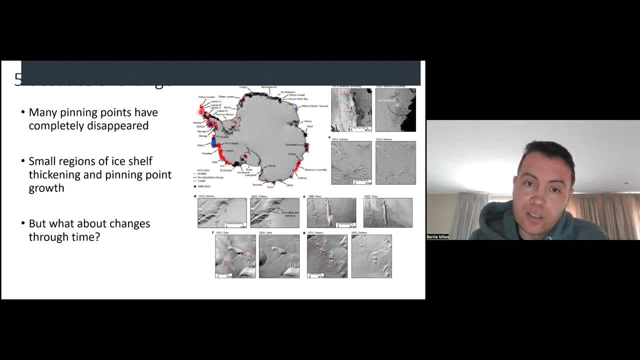 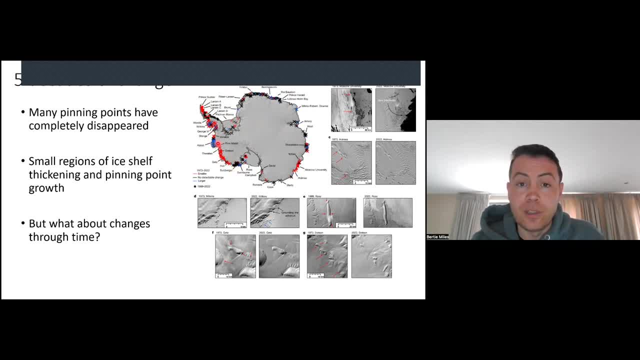 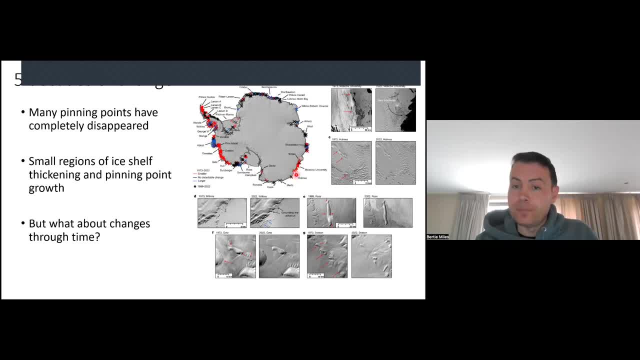 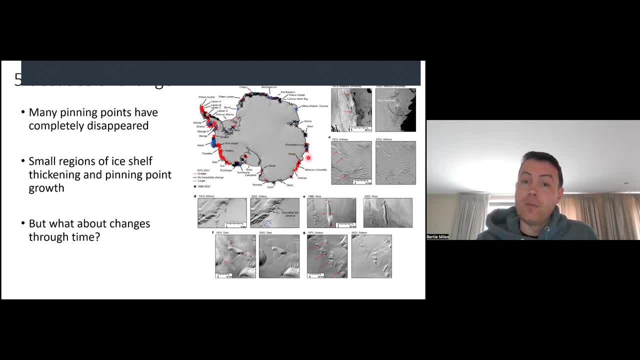 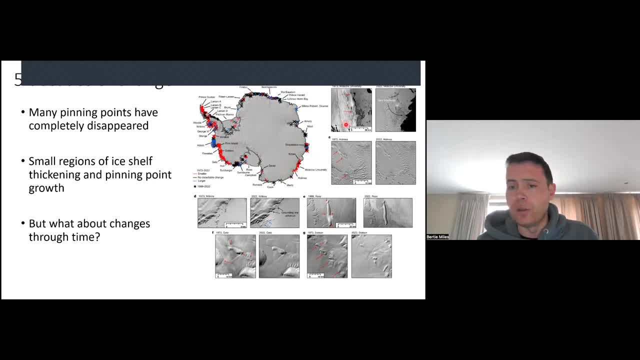 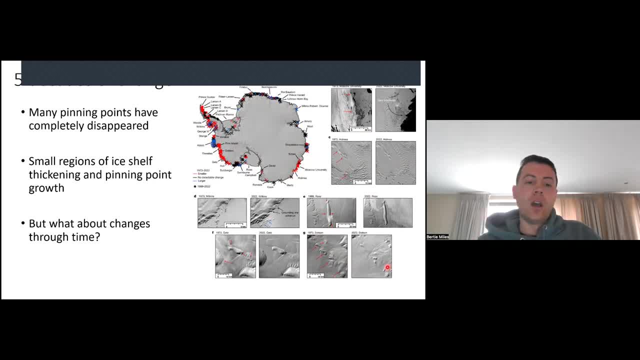 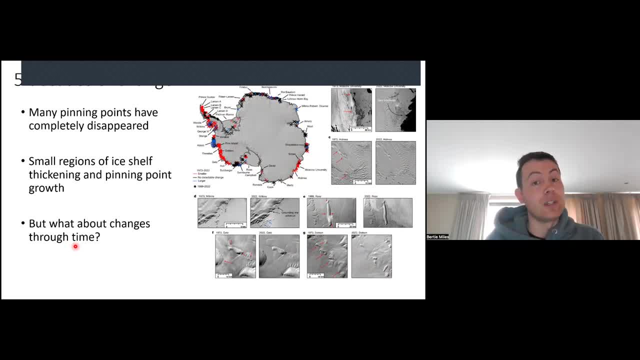 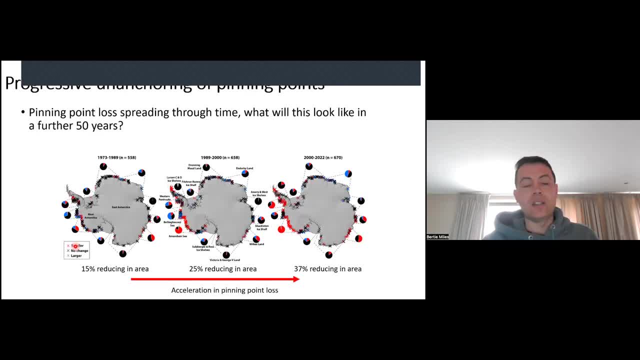 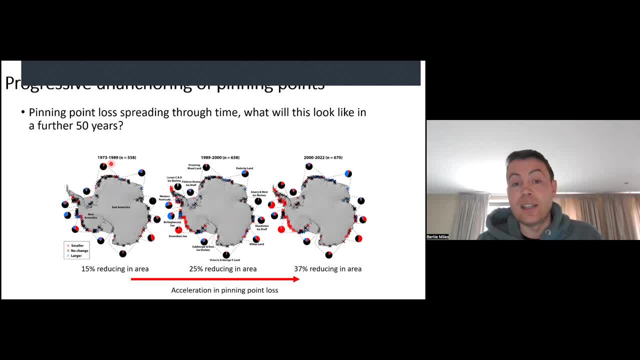 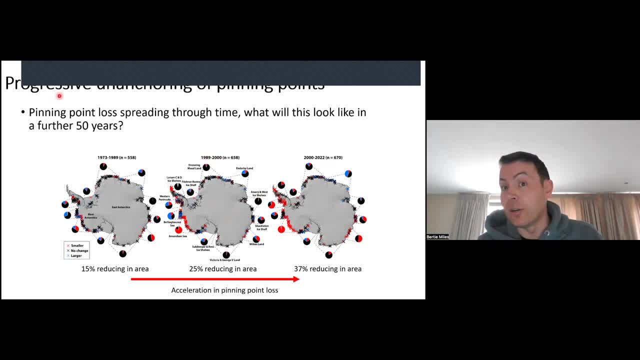 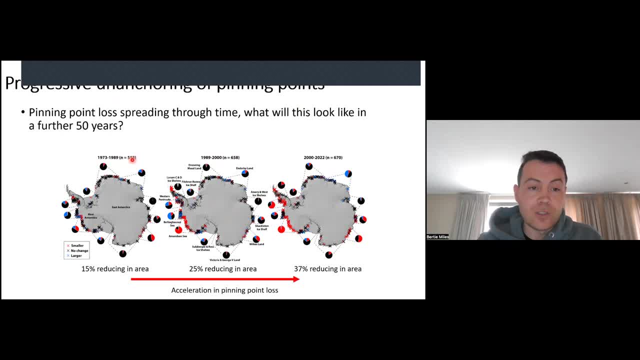 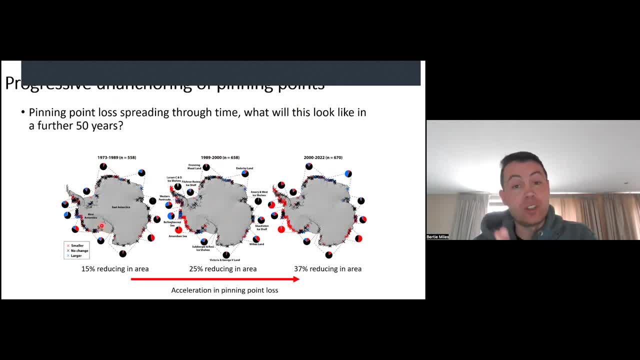 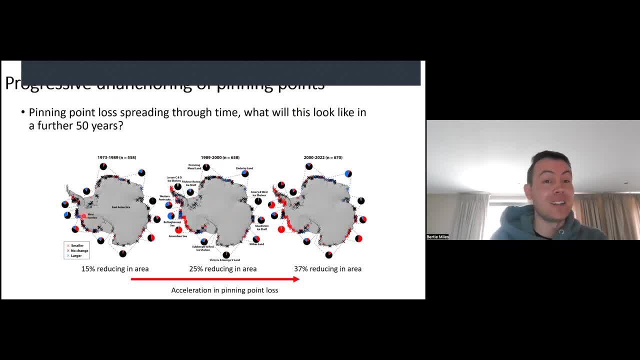 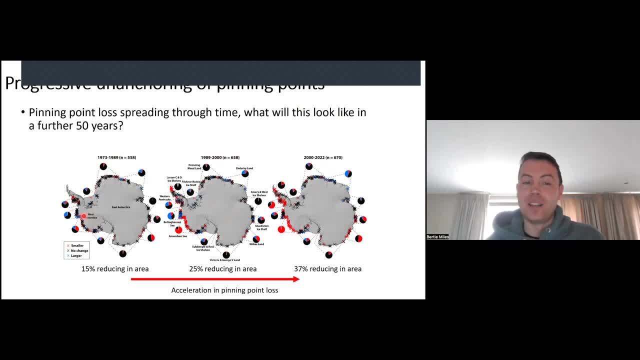 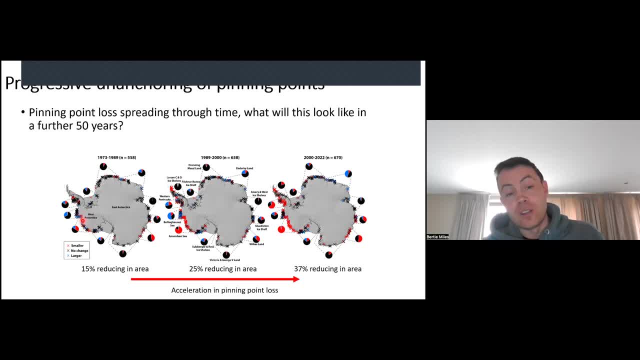 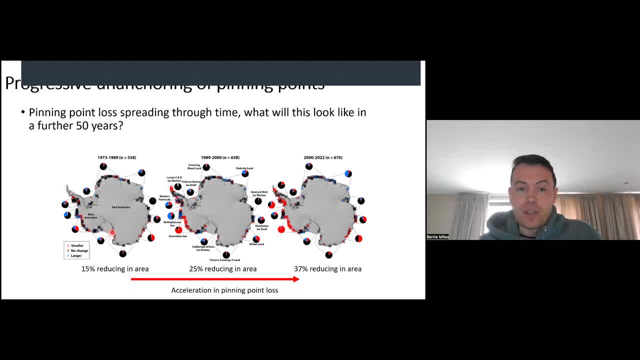 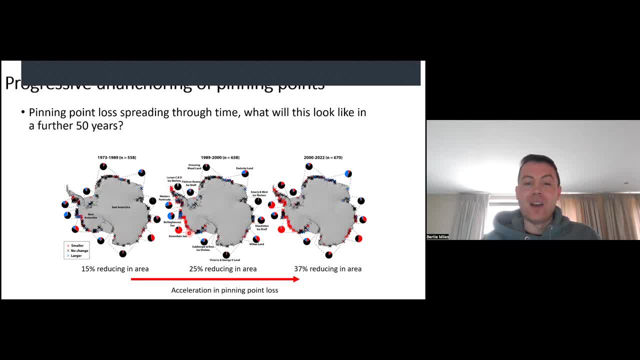 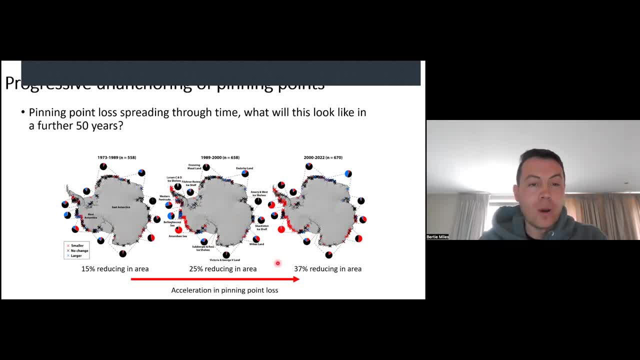 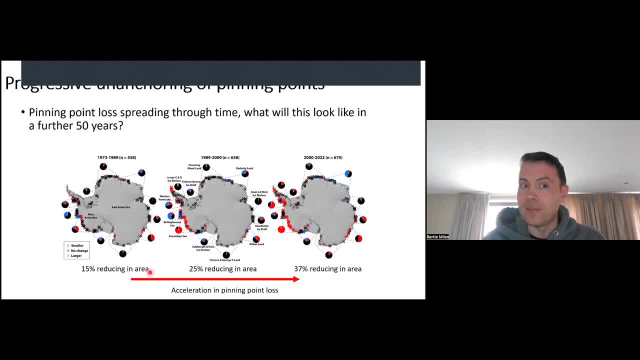 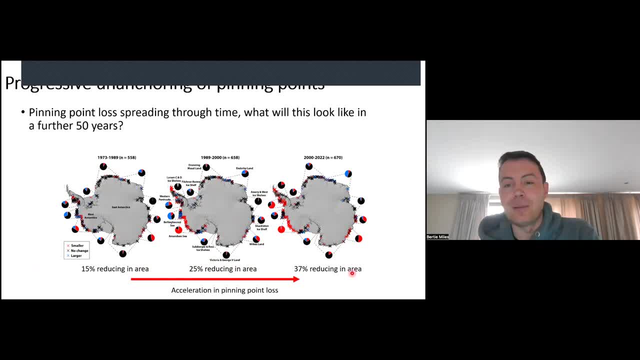 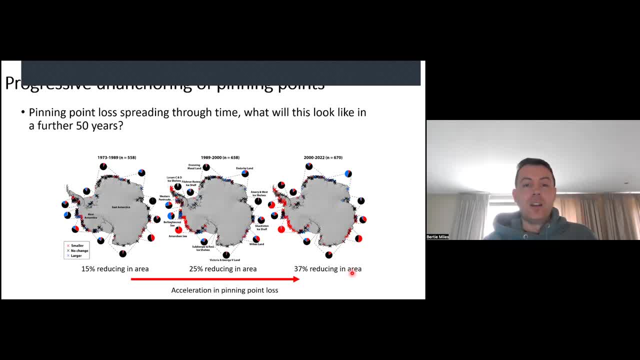 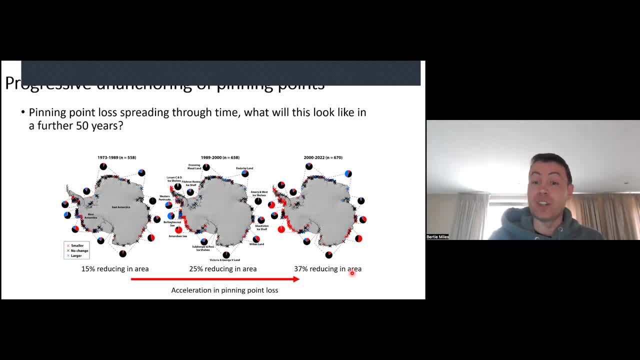 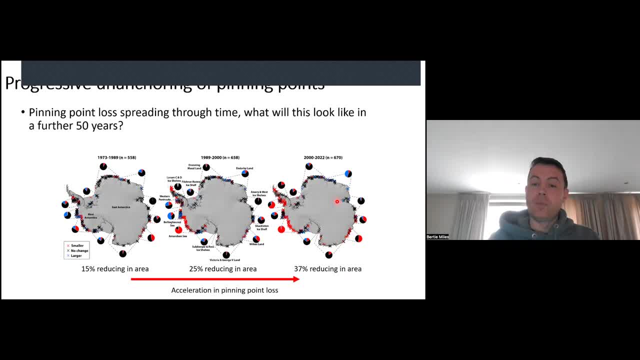 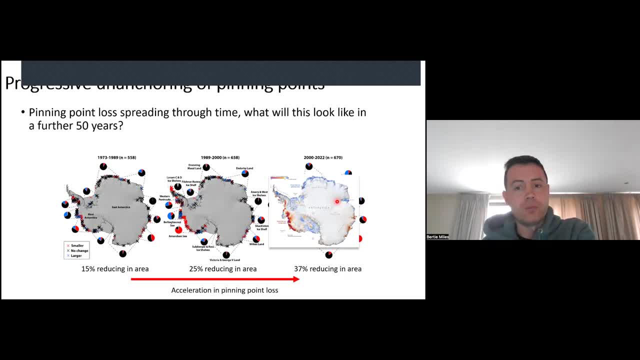 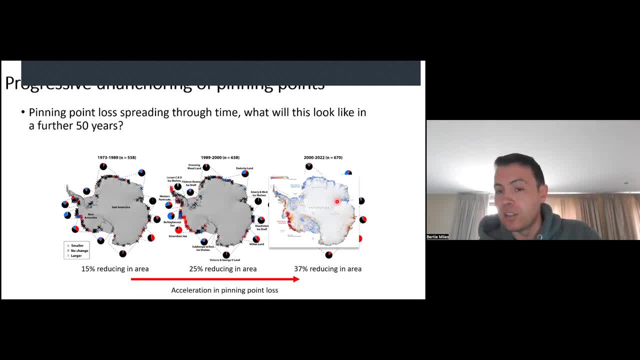 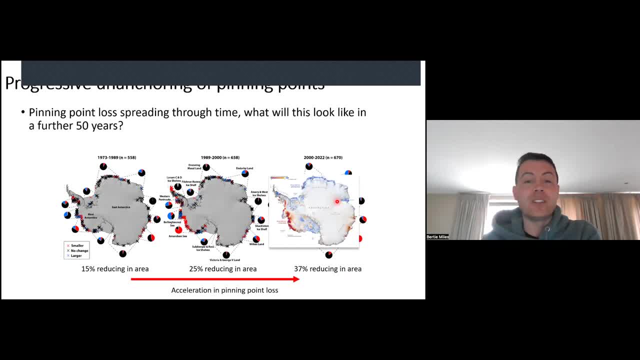 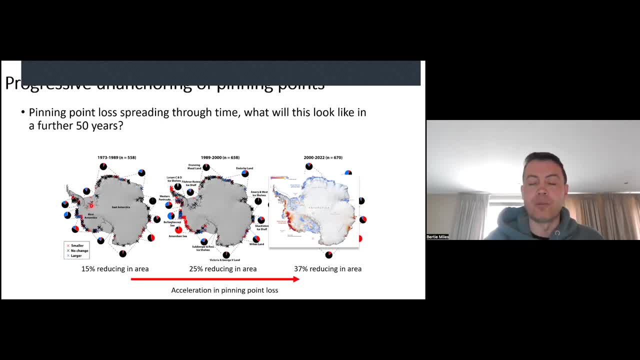 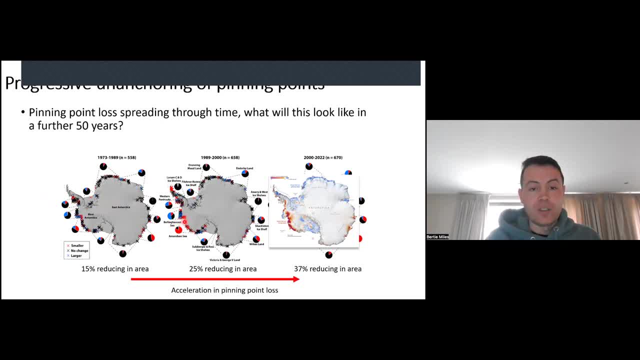 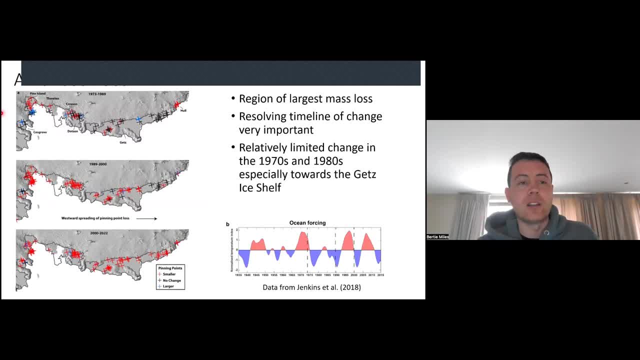 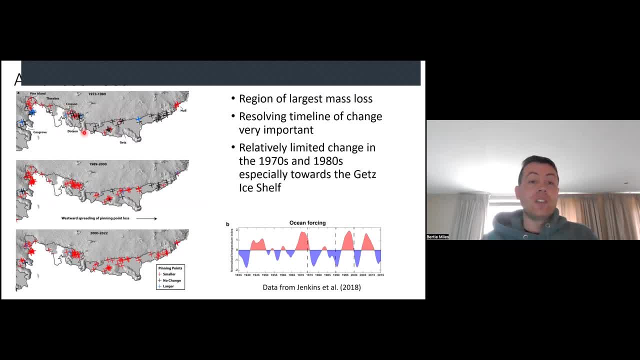 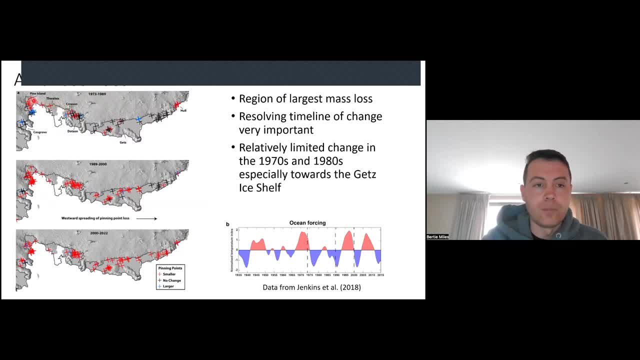 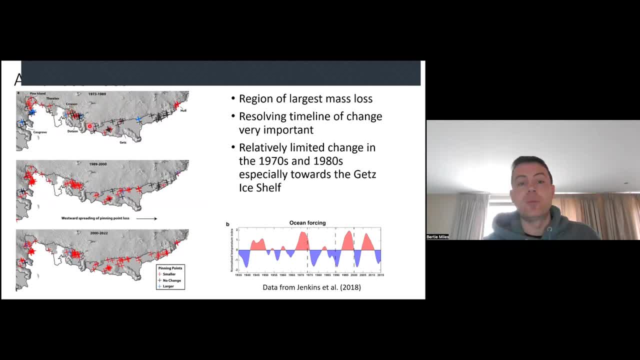 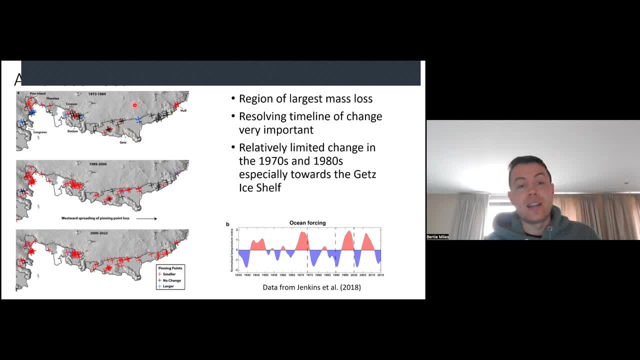 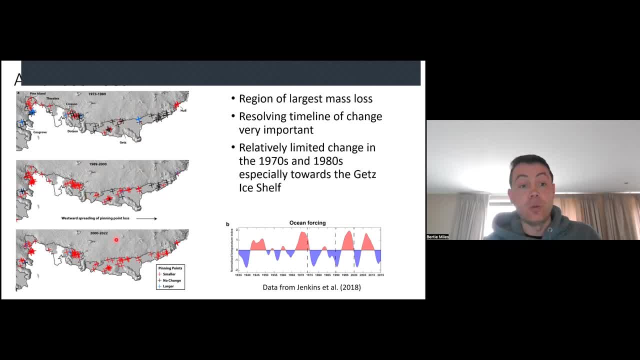 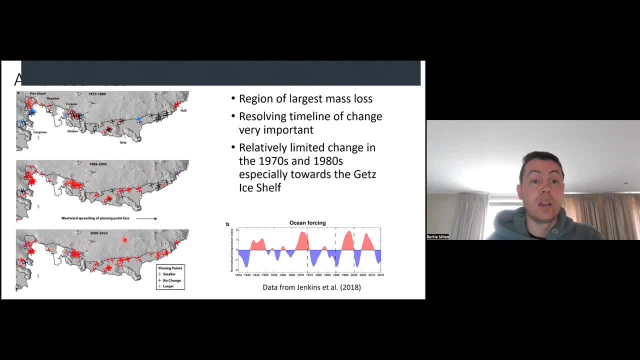 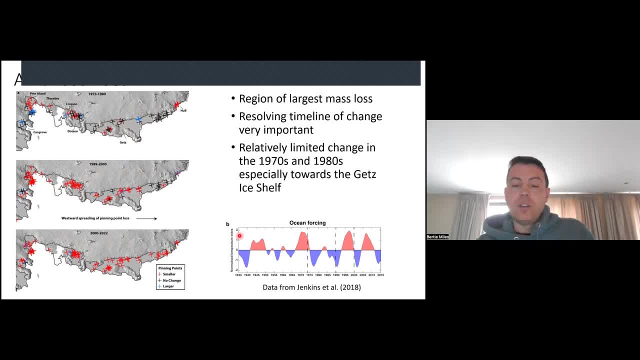 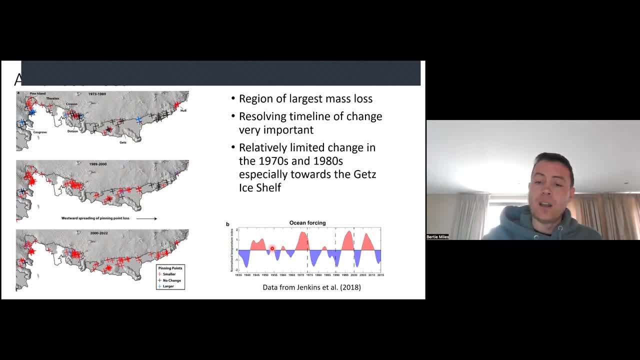 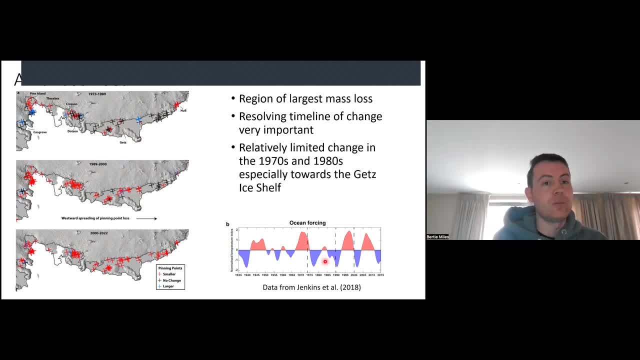 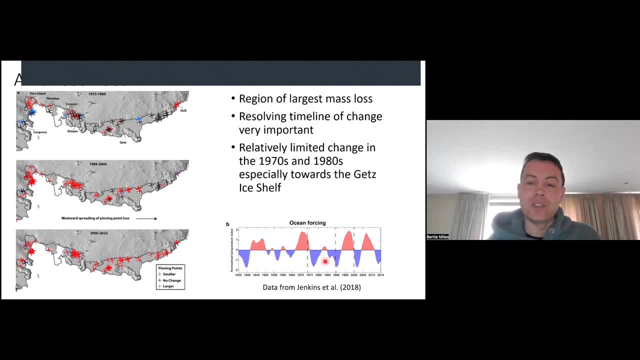 University And what it's showing is that this is a series of radar images made by Adrian Lockman at Swansea University, And what it's showing is that this is a series of radar images made by Adrian Lockman at Swansea University. we can see that the 70s and 80s may be likely relatively cool period. 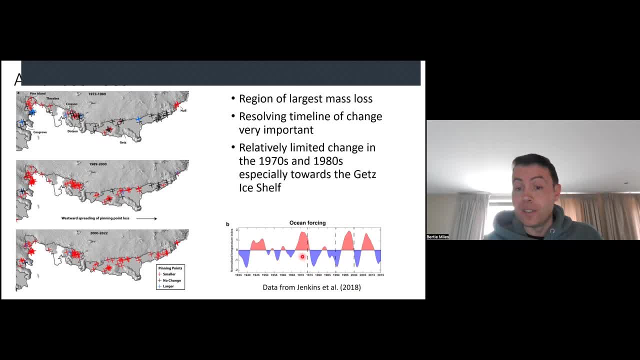 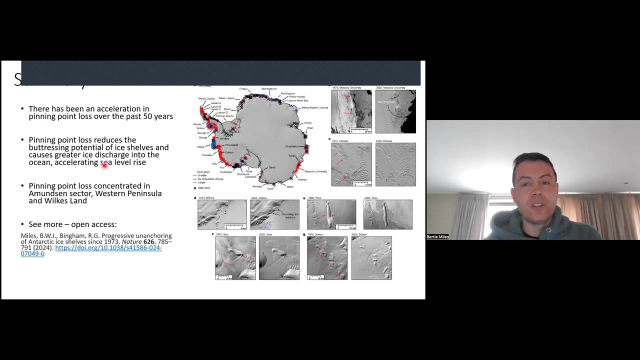 so if we had imagery in the 1960s and capture this kind of warm spike, it may have looked slightly different. so, in summary, there's been an acceleration and pinning point loss over the past 50 years. and why this is important: we don't just bump some of the surface, but important because we 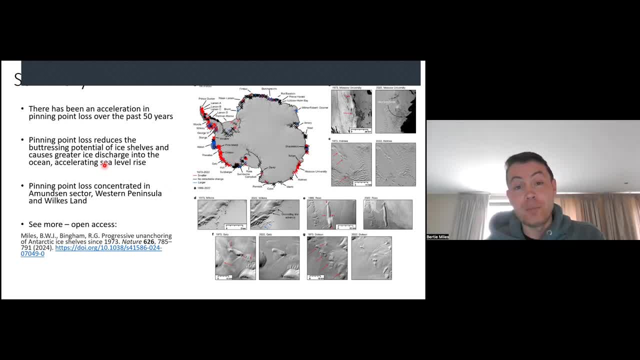 provide this buttressing. so, because we've got this acceleration pinning point loss, the buttressing is reducing and that means more ice is being discharged into the ocean, which is causing sea level rise. and this pinning point loss is largely concentrated in west antarctica, the western peninsula and in the wilkes land section of east antarctica. 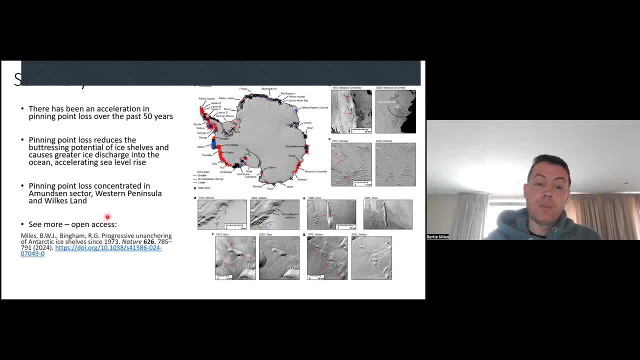 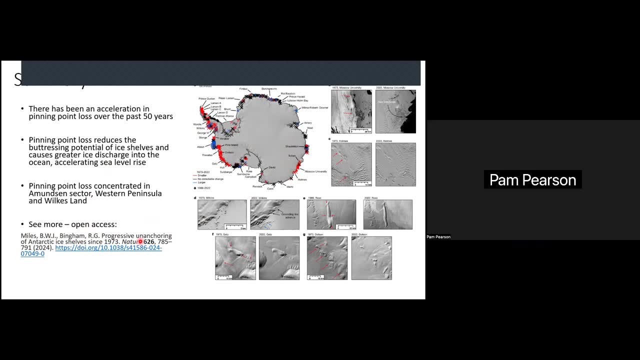 and, if you're interested, you can see more in our paper, which is open access, and i've just put the link below that. so thank you very much. thank you so much, birdie. um, are there any questions? and simply raise your hand, or or start speaking, or uh go ahead and and uh put on your video. 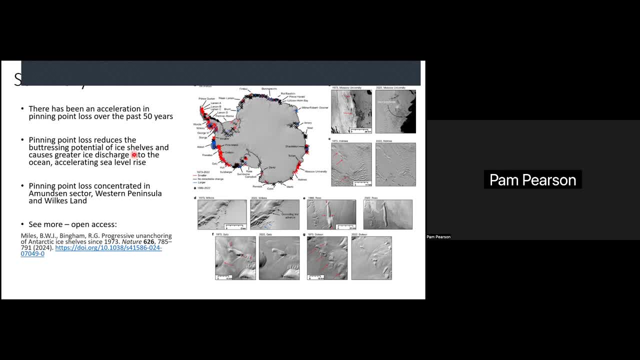 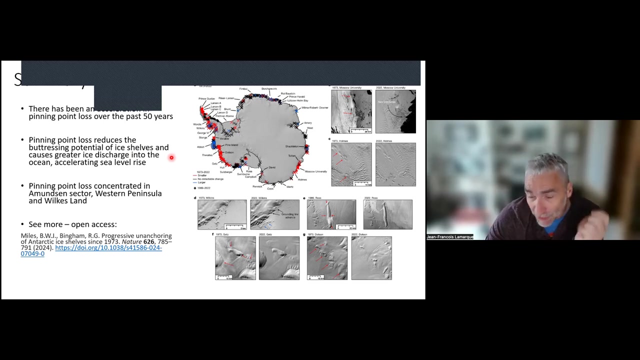 len, did you have a question? yeah, jean-francois, please go ahead. hi, um, birdie, thank you. this was, this was great, great presentation. um, fortunately i could only join partially through, so this might be a question you've you've answered before, but so in in the. 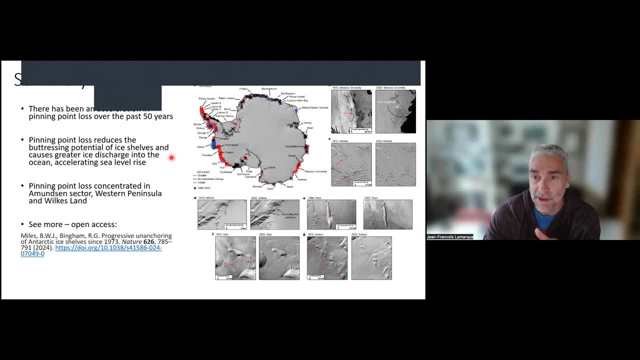 early part. you, you mentioned that how difficult it was to use landsat to come up with with pictures. so is. is there a risk that your um, or the early part of your analysis, is uh, confronted with just in turn in your annual variability or decadal variability? because you know, you're, you're not? 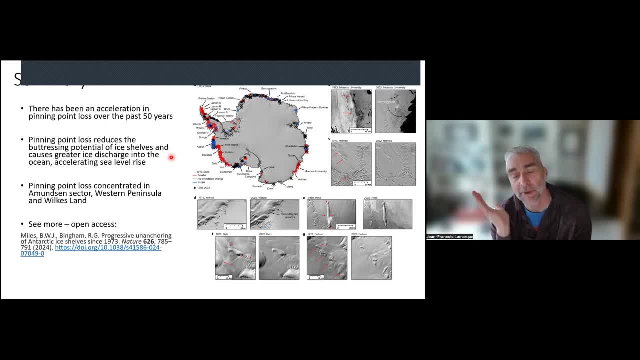 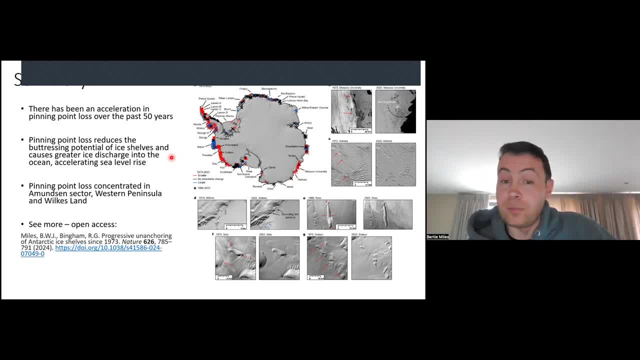 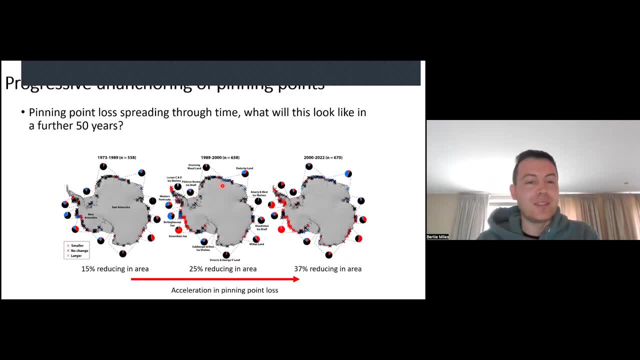 yeah, it's this. thank you for a question. um, i would personally say it's very much a trend. maybe this is probably the best figure to show this, but you can kind of see this in the 70s. you're starting to be maybe a little bit of red, particularly in this western antarctica region, as you get to 1890. 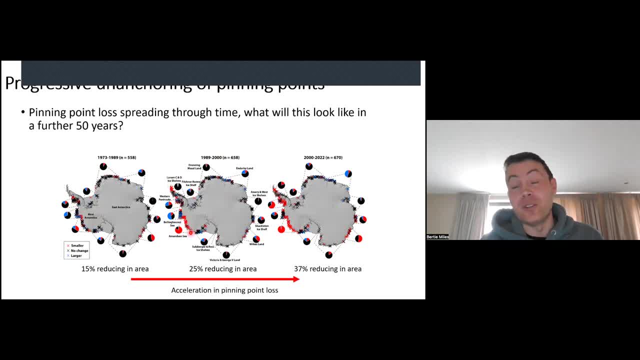 you can see, it's slowly spreading a bit more and again. when we get to 2000 it's almost covering this entire 3000, 4000 kilometers stretch of coastlines. you can really see this, this pinning point loss, spreading, and the reason that is is because progressively, more and more warm water. 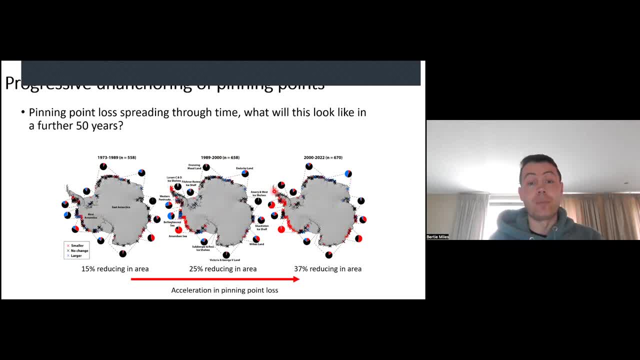 is coming and melting the underside of these ice shelves, right. so my point was was mostly: how many? when you, when you look at 1979 to 1989, are you fitting a trend line or just looking at the difference between the, the, the two end points? it's basically 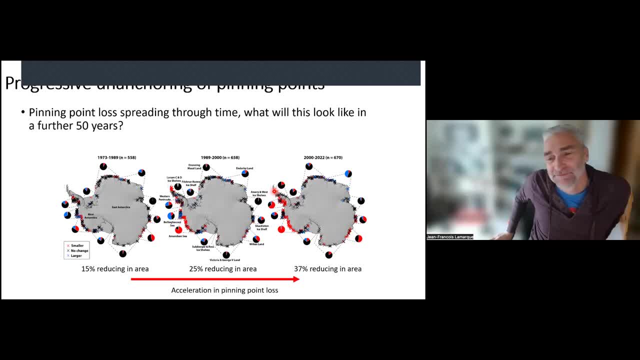 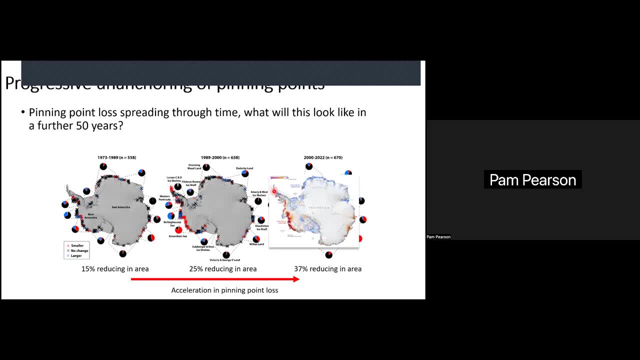 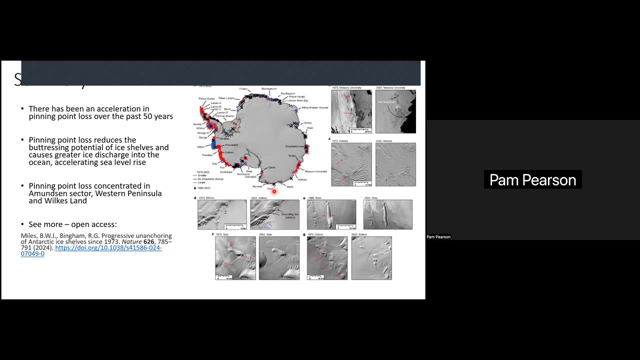 difference between two points in time. okay, okay, thank you. any other questions and we'll? we'll have a time for, for, uh, new questions also at the very end. um, but otherwise seeing nothing, we'll go ahead then and uh, thank you. so much, birdie, and you can take. 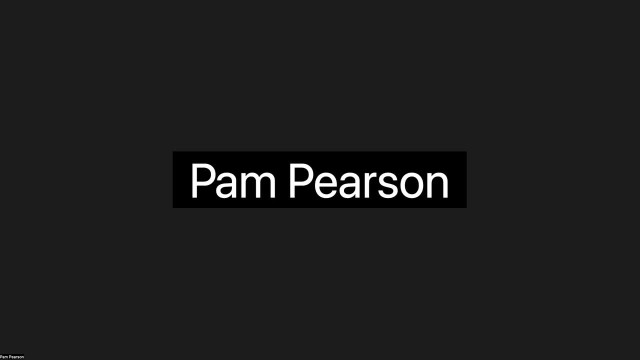 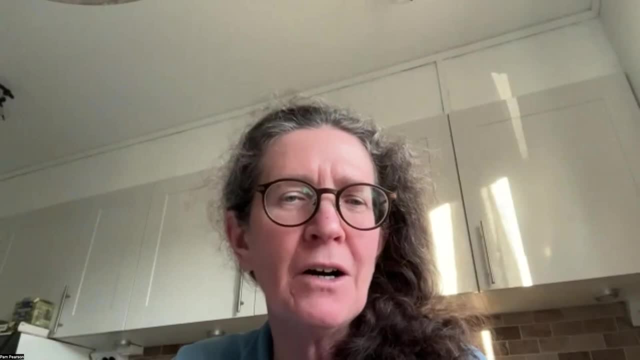 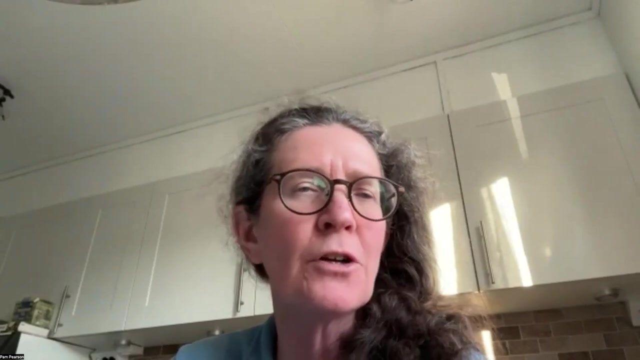 your slides down. and sean pryor, who, uh, just recently came back from the ppr imo meeting, uh, where there was quite a bit of focus on, obviously, a variety of ship pollution issues, but in particular, uh, i asked her to maybe address some of the the progress, or lack thereof, of black. 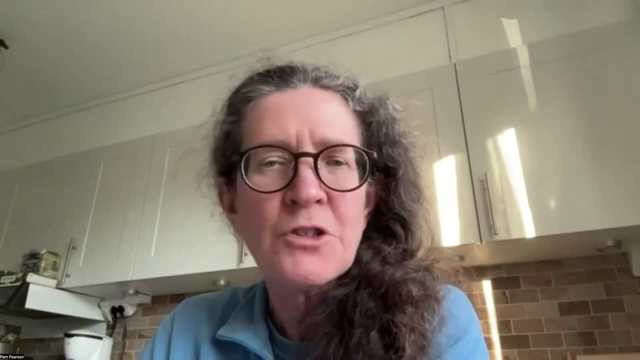 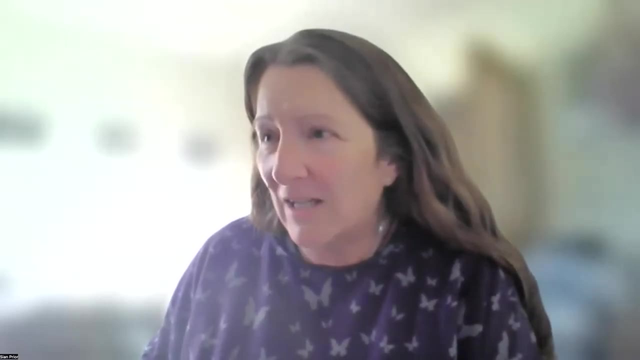 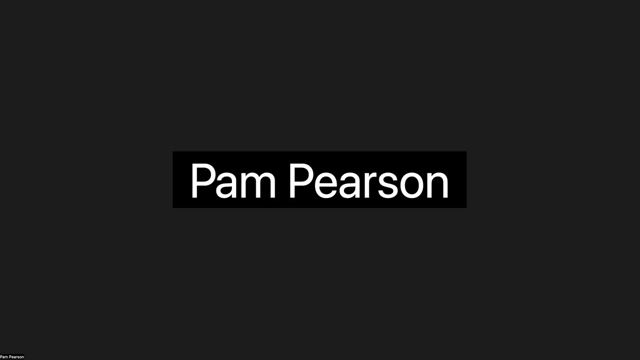 carbon, um, so please go ahead, sean. thank you, pam, and thank you for uh inviting me to come and speak today. i can't actually share my screen. it's saying host: disabled participant screen sharing. let me try again. you should. you should be a a co-host, which should make it possible for you to. 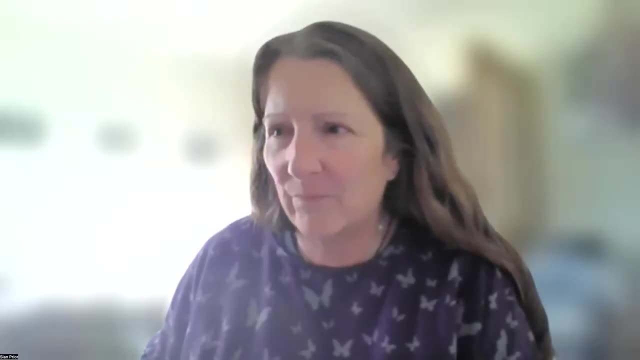 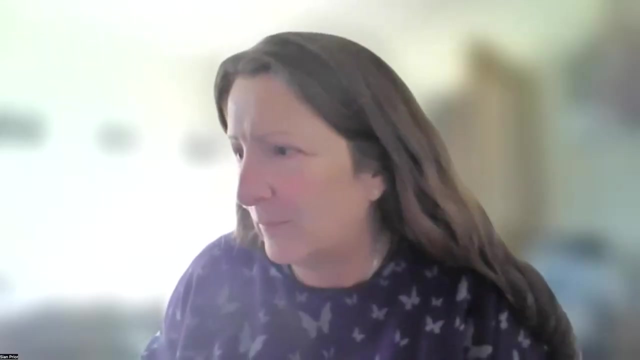 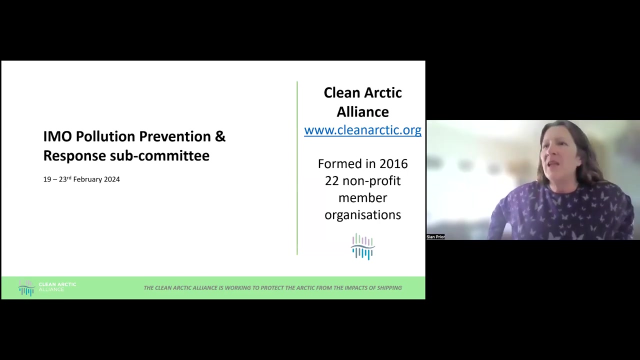 screen share. if not, i can do it right now. never mind, you got bumped out as co-host, now go ahead. okay, there we go. sorry about that, that's okay, no problem. hopefully you can see my screen now sharing the right one as well. let's just make sure it works. no, it doesn't okay. 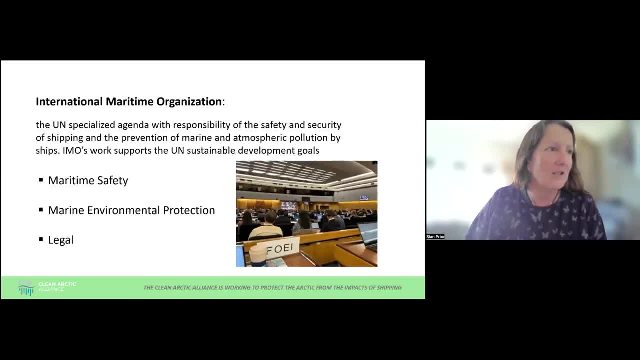 okay, um, as pam said, i've recently returned from um the international maritime organization discussions of one of their um technical committees. perhaps, just before i get into that, i'll just take a step back and just remind um or just summarize how, how the imo works. the imo or international maritime organization. 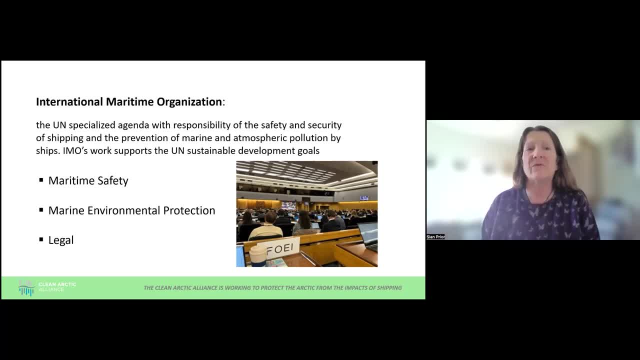 is the un specialised agency which is responsible for safety and security of shipping, and i noticed recently they've added to their remit um the prevention of marine and atmospheric pollution by ships. um, they've been working on protection of the marine environment for certain- uh, almost home. 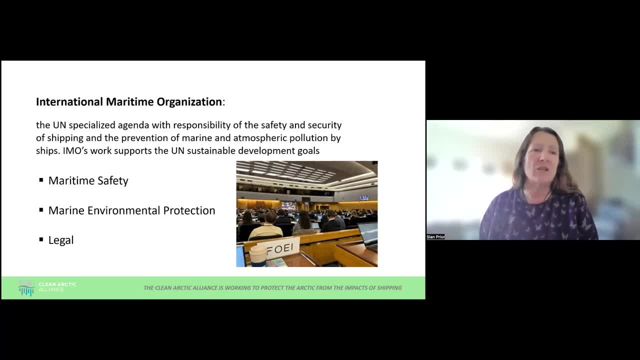 marine environment for well since its inception, but i think safety was always seen as the higher priority, but there is now so much happening in terms of prevention of marine and atmospheric pollution that it's seen as pretty much an equal priority. um, they have three, uh, what they call. 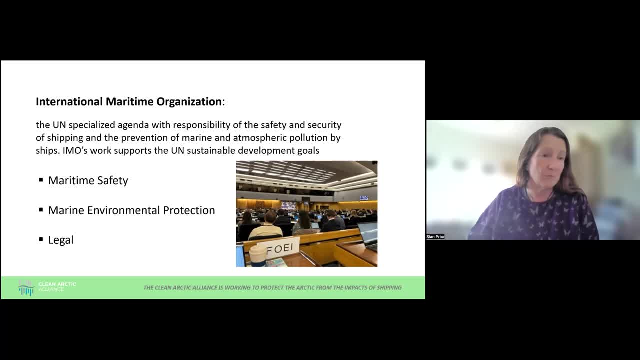 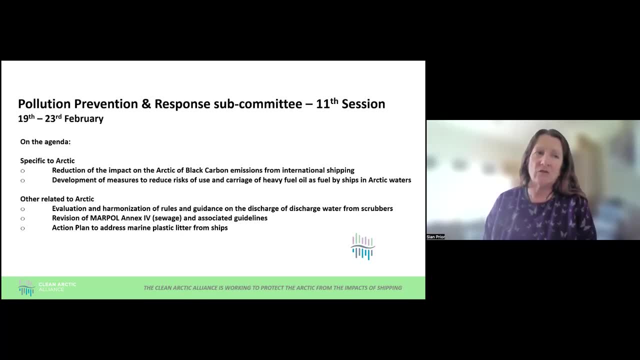 mother committees: the maritime safety committee, the marine environmental protection committee and the legal committee. but what i've just been at two weeks ago is the pollution prevention and response subcommittee. this is one of the technical committees that reports to the other committees, particularly to the marine environment protection committee, but also to the safety committee as well. 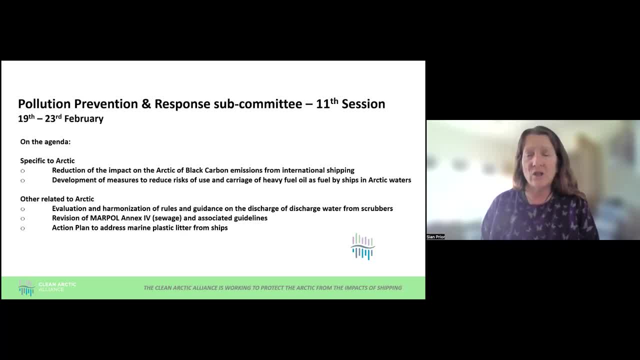 and it had its 11th session two weeks ago, and on the agenda were two items that were specific to the arctic: uh consideration of the reduction of measures to reduce the impact on the arctic of black carbon emissions from international shipping, and also the development of measures to reduce the 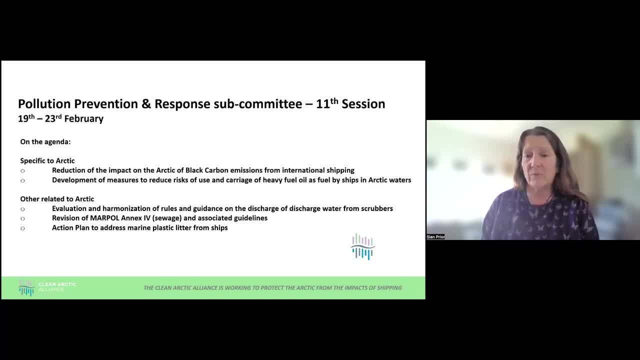 risks of environmental pollution in the arctic, and also the development of measures to reduce the risks of use and carriage of heavy fuel oil as fueled by ships in the arctic. and then a number, a whole range of other issues, some of which are related or have relevance to the arctic and protection of the 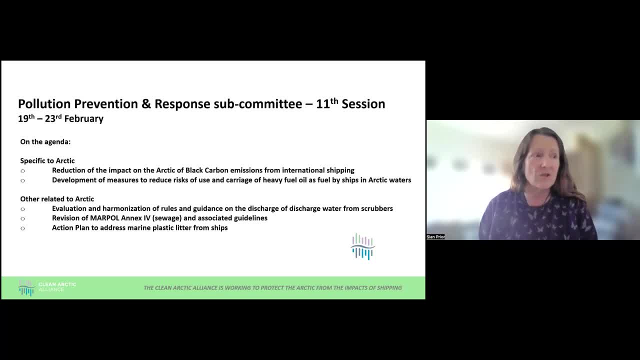 arctic and i've highlighted just three here that we focus on: um the uh rules around the use of scrubbers and the discharge of scrubber waste water. um rules around um how to manage sewage and sewage emissions from ships. and marine plastic litter. i'm not going to go into a 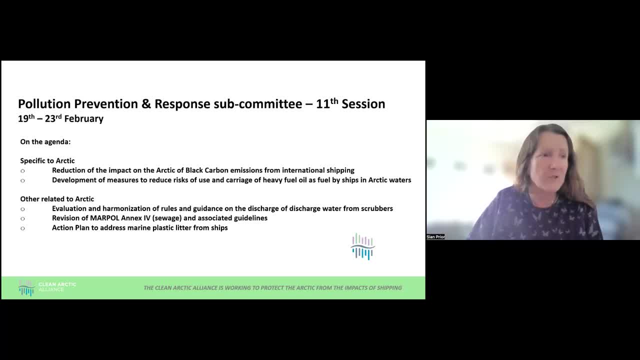 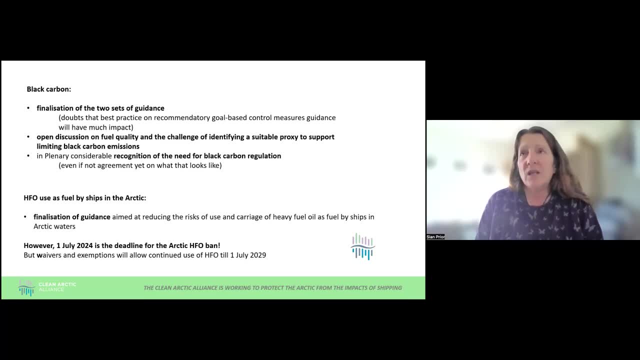 lot of detail on all of them. i'll focus mainly on the ones that are specific to the arctic um. in terms of the overall meeting um, at the beginning of the meeting we issue a press release on what we hope to see come out of the meeting for the in the during the week, and then then, at the end, 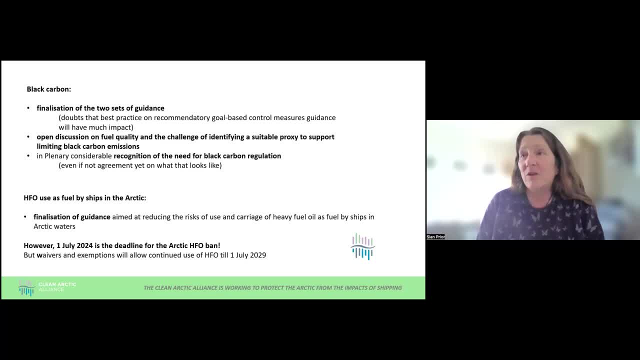 of the week, we issue a press release saying: you know how we feel the meeting has gone and, as usual, i think our press statement at the end of the week was somewhat frustrated that there hadn't been more, that there hadn't been more achieved, um, but having said that, i think there was progress. 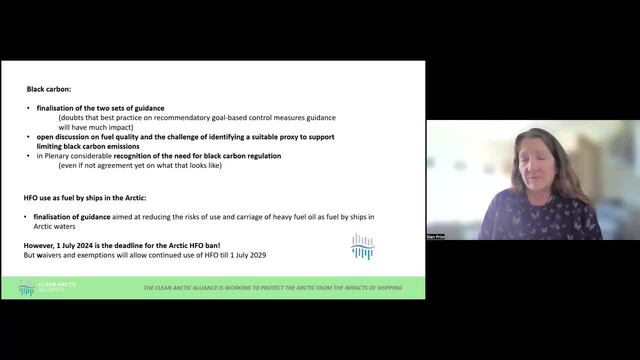 on certainly two of the issues um that are of greatest priority for us and of relevance to the arctic, but not enough, not nothing that was leading to really tangible um regulations in the future. so our press release was was somewhat middle of the road this time and and wanting to see more progress, but what we did achieve, or what was achieved. 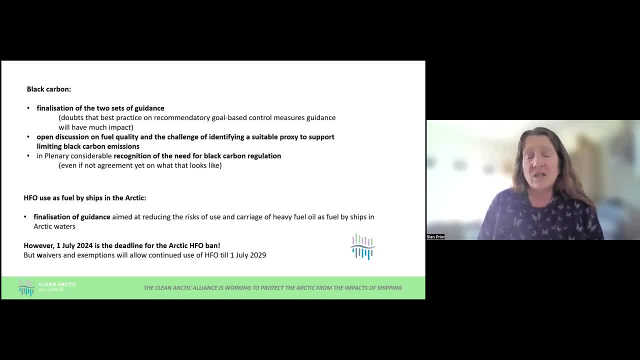 on black carbon. this time was two sets of guidance, two new sets of guidance, one looking at best practice um and the other one looking at the measurement and monitoring and reporting of black carbon emissions. the best practice guidance is seen as an interim measure and i think good for the first time was the fact that it really was seen as an interim measure. 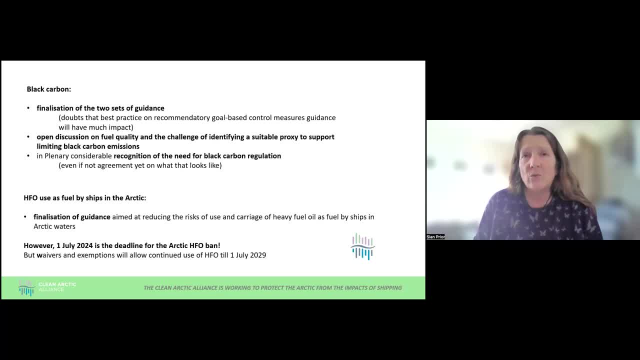 there was a lot of talk around the need for regulation, which hasn't happened. in the past, there's been question marks around whether regulation of black carbon emissions is actually needed. um, but this time you know the the best practice guidance was finalized. it won't be approved till later this year, but it was finalized, um there are concerns. 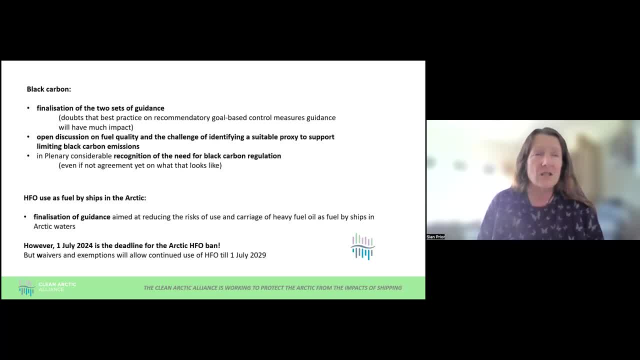 though, is whether it'll really have a lot of impact, because it is guidance and it's on best practice, on recommendatory gold-based control measures, and what this means is that ships and shipping companies will be able to decide for themselves what they're going to do to try and 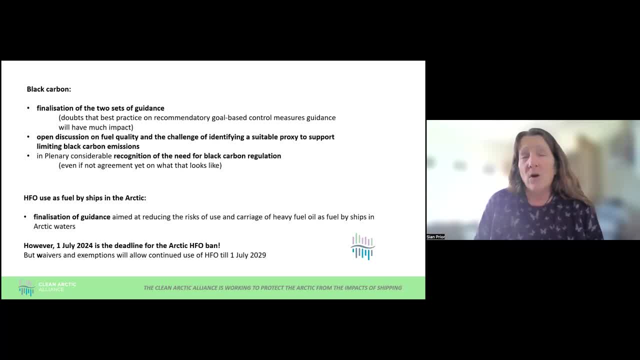 actually reduce black carbon emissions. hopefully it will have an impact, but we? um are doubtful, because the history of guidance from the imo is not great. um it tends to be deprioritized compared to regulation and often shelved, so we're not holding our breath on that. um what was good, though. 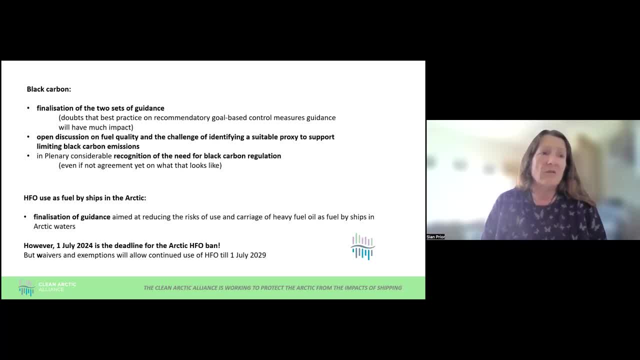 was that for the first time, there was open discussion of issues around fuel quality, and the fact that it is the fuel is just an issue, and there is a great deal of uncertainty, but we've received good media reasoning and information from other countries and we're working in. 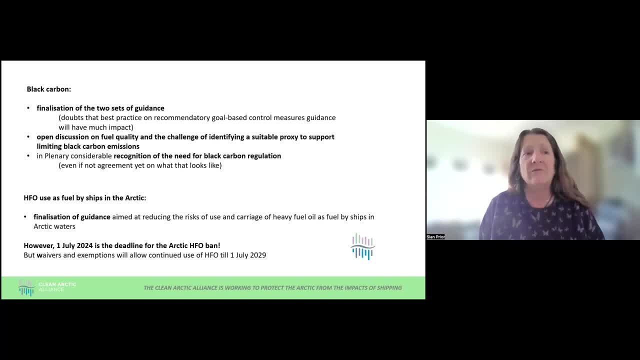 many different places on the issue of fuel quality and diesel soul, and these issues are a very important factor in our thinking about the pressure of fuel, which is one of the things we looked at in our last study, which was the need for a more coordinated approach to fuel to fuel. 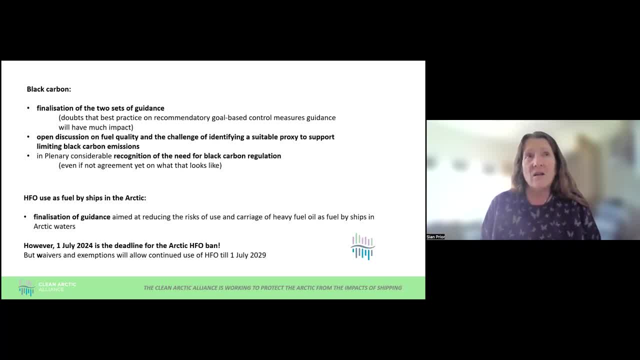 refueling and diesel fuel consumption and fuel production, and that's one of the things we looked at. fuel being used and the proportion of aromatic versus paraffinic components in the fuel makes a big difference in terms of black carbon emissions. but what is challenging is how to. 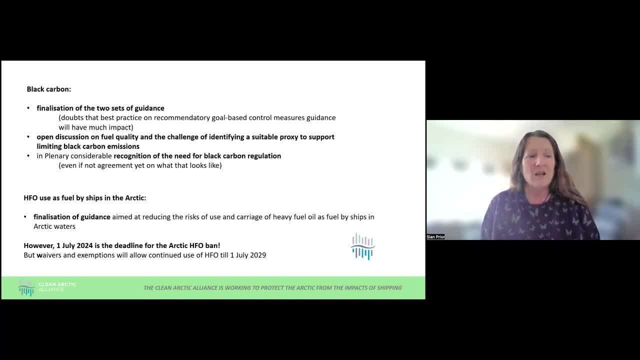 determine before it's burnt what black carbon emissions are different. each different type of fuel oil that is available to shipping is going to produce in terms of black carbon, and there was a very open discussion at this meeting, both in cleanery, in a side event that we organized, and in a working group, of these issues and, although not a lot of progress at this, 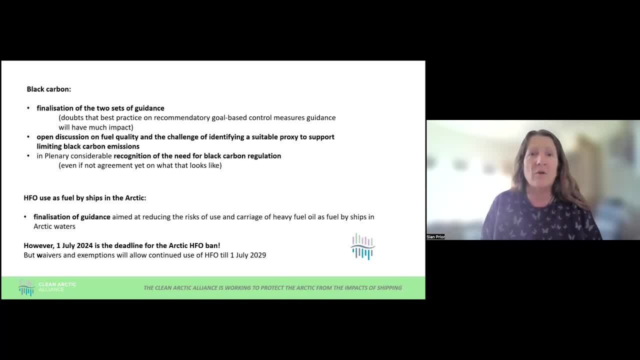 point. certainly, I think the issues are out on the table and people are minded to try and get to the bottom of this and, as I say, you know, in cleanery particularly, there was, I think, good recognition of the fact that ultimately we need black carbon regulation and actually I, you know, I find it. 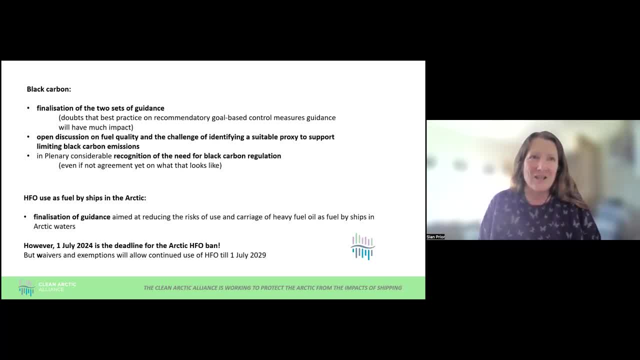 amazing in this day and age that there is a sector for which emissions of black carbon are short-lived- a very potent, short-lived climate force- that are still unregulated. moving on to the guidance on heavy fuel oil use in the arctic, the guidelines, or the guidance, was finalized and it will be adopted. 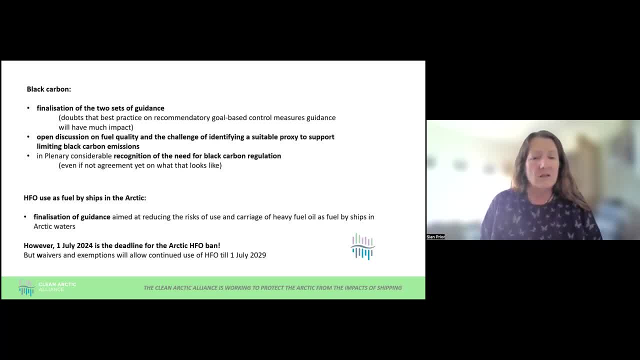 later this year we didn't get terribly engaged in this discussion. the work's been around for a few years. it's taken a little while to reach finalization and to some extent we're hoping it's somewhat overtaken by events in the from the first of July this year and we're hoping that. 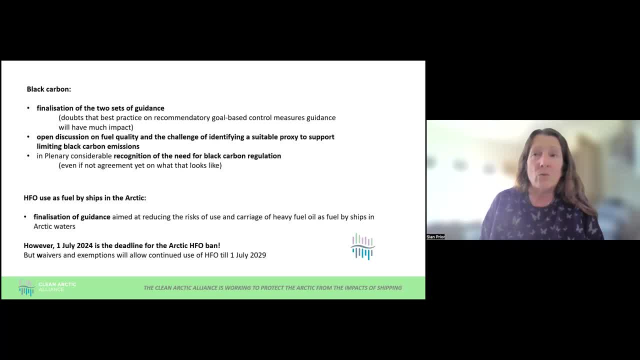 this year there is a new regulation that will start to take effect that will actually require ships not to use or to carry for use heavy fuel oils, which are the most polluting fuels, have the highest levels of black carbon emissions in the arctic. having said that, and where the guidance 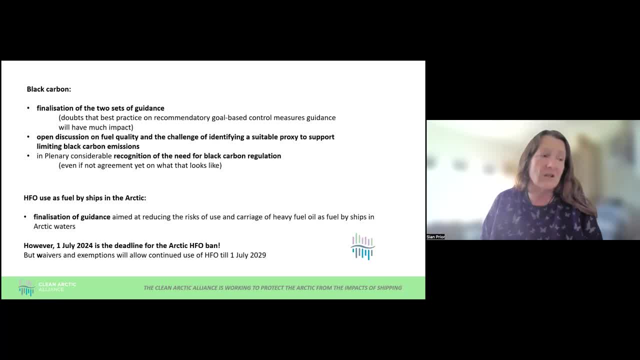 probably will be valuable is that, although the regulation takes effect from the first of July, there are waivers allowed and exemptions depending on the structure of a ship and whether its fuel tanks are protected. so that's where the guidance will come in, but ultimately we want to see shipping moving away. 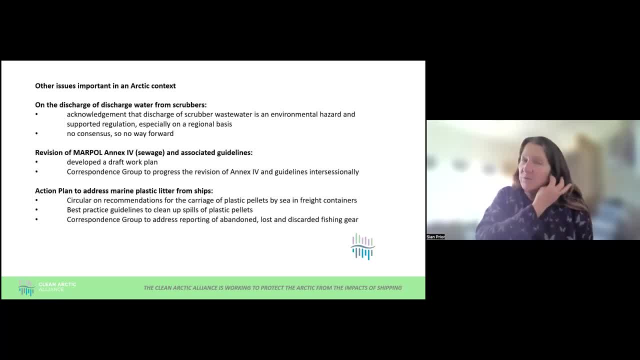 from using these dirty fuels. there was progress on some of the other issues. scrubbers is one that is particularly important to us. scrubbers are used to allow ships to continue using the older, dirtier fuels that have been not banned as such, because they can still be used, but the amount of 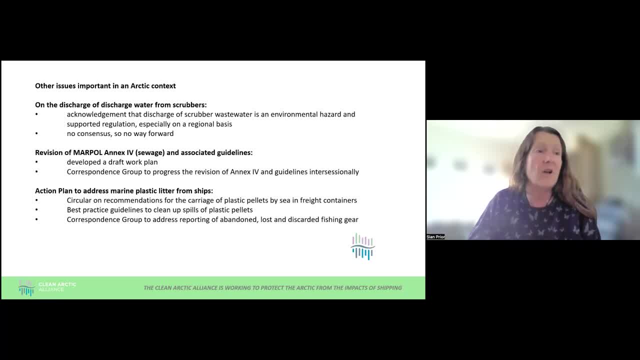 sulfur in the fuels has to be reduced and the amount of sulfur in the fuels has to be reduced, but to allow the use of high sulfur fuels, ships can install scrubbers and still extract the sulfur after the fuel has been burnt from the exhaust. unfortunately, most of the scrubbers are what are. 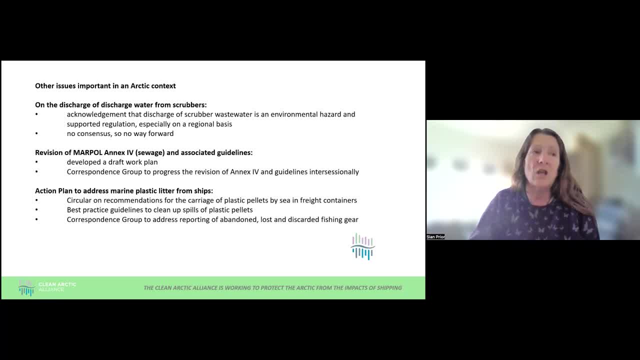 called open loop scrubbers and these a lot of seawater to wash the scrubber exhaust to remove the sulfur, and that waste is then dumped back into the ocean which brings with it ocean pollution, problems with polyaromatic hydrocarbons, heavy metals, nitrites, nitrates and other. 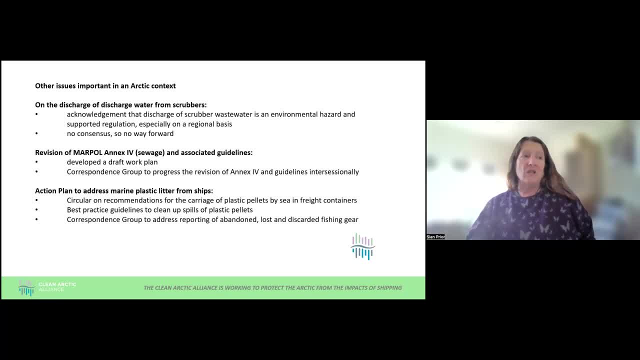 ways as well. what was good at the meeting two weeks ago was that there was a good acknowledgement- though not by everybody yet- that this is a problem, an environmental hazard, and it needs to be addressed. there was good support for addressing it, not globally, unfortunately, but on a regional. 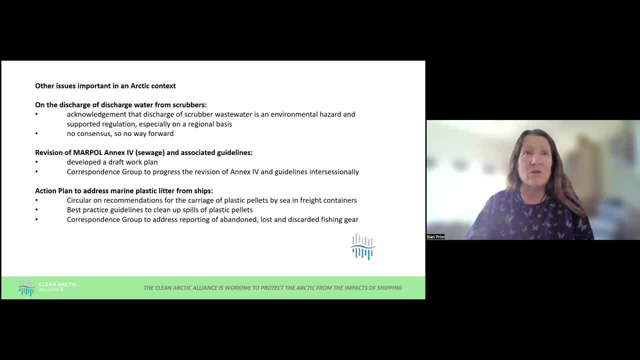 basis at least. however, there was no consensus around how to move forward on this, so unfortunately there's no steps identified to move forward at the moment, but countries have been encouraged to come back to the next meeting in a year's time with some proposals for ways forward: sewage and litter quickly. there was a little bit of progress. 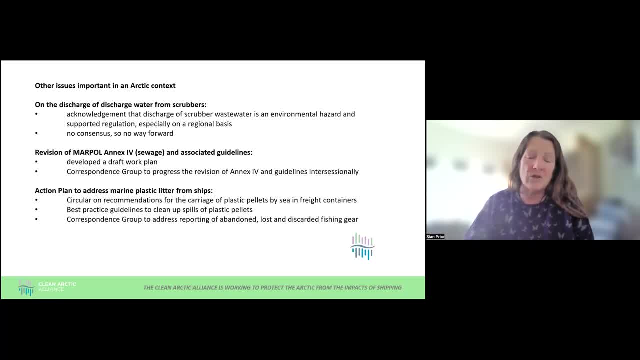 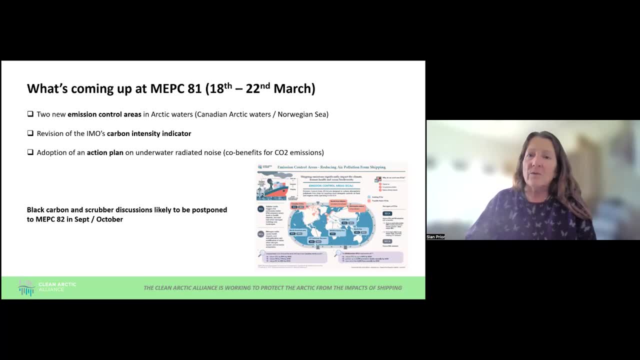 in both areas. but most of the work, or a lot of the work that's of particular interest to us, is going to be sent to correspondence groups that will work intercessionally. so that was ppr, it was only two weeks ago, but we now have the mother committee, the marine. 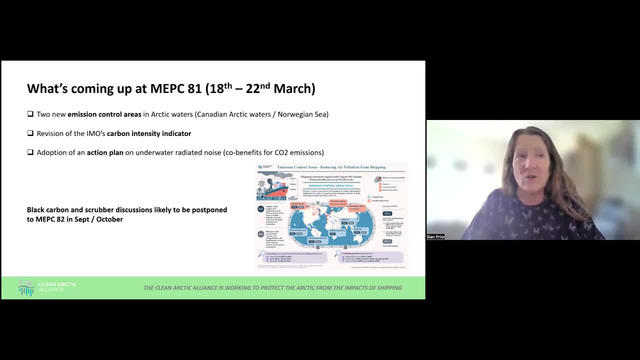 environment protection committee coming up in 10 days time, or less than that now, a week after next, and on the agenda here there's going to be more that is of relevance to the Arctic. There are proposals for two new emission control areas in Arctic waters, one covering Canadian Arctic waters and one covering 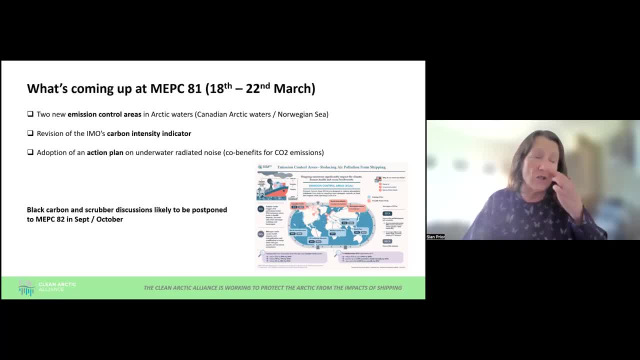 the Norwegian Sea. These measures, or at least these designations, will control emissions of sulfur and nitrogen, so, SOx and NOx in these waters and will be important for the protection of the Arctic environment. There will also be a discussion of global efforts to reduce greenhouse. 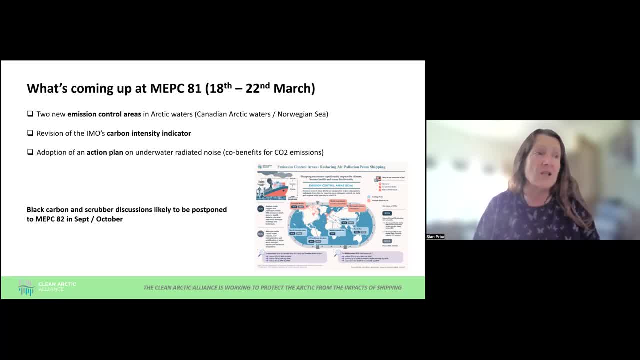 gas emissions and, in particular, revision of the existing carbon intensity indicator, which at the moment is really not much better than business as usual, but there is a commitment to strengthen it, to start making it more effective in reducing shipping carbon emissions, And also there should be, hopefully, adoption of an action plan. I'm not sure if it's a good idea to do that. but I'm not sure if it's a good idea to do that. I'm not sure if it's a good idea to do that. I'm not sure if it's a good idea to do that. 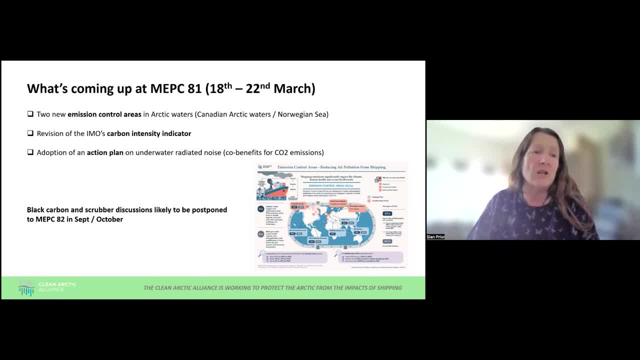 underwater radiated noise, which again is important in the Arctic context, not just because noise is a relatively- or shipping noise is a relatively new phenomenon there, but also because, by reducing underwater radiated noise, depending on the measures used, there will be co-benefits. 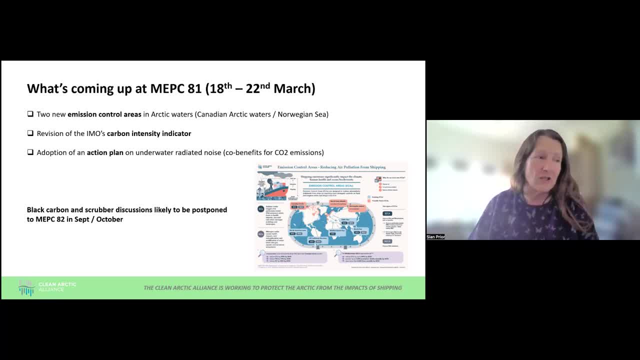 for CO2 emissions as well. Unfortunately, because PPR and MEPC have occurred in close proximity to each other, a decision has been taken to postpone any further discussion on black carbon emissions and scrubber discharges to the next meeting of the Marine Environment Protection Committee. 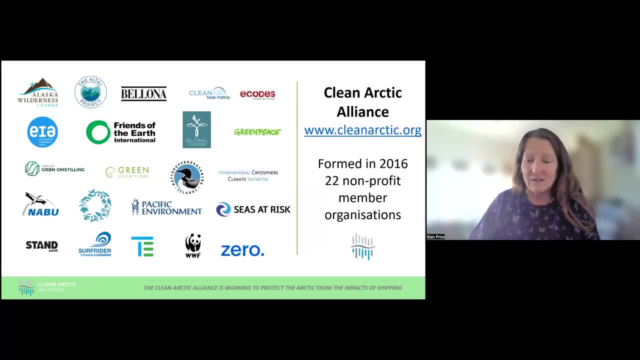 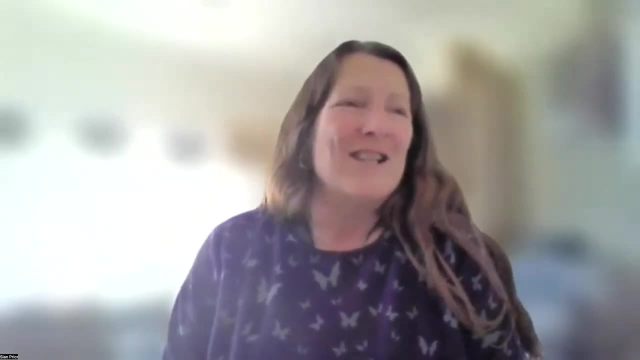 which will be later this year. And that is it. So sorry, very brief and very quick. Thank you so much, Sean, and congratulations, at least, on getting the fuel issues on the table. That's progress. It is Slowly, slowly getting there. 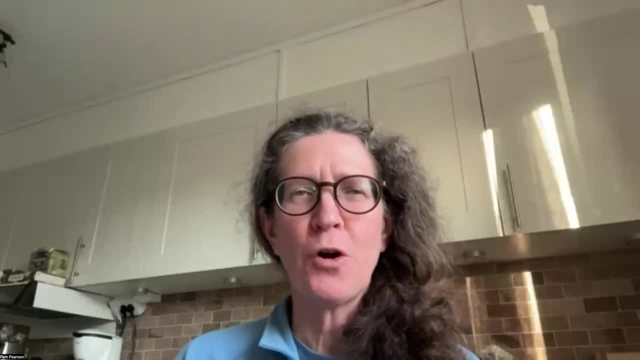 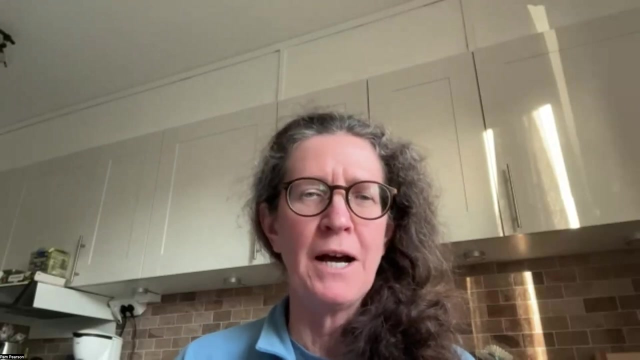 If there are any questions for Sean or Bertie or Julia, everyone should feel free to turn on their videos if they wish And please ask your questions. We certainly have a couple of minutes until the top of the hour, but I can go on, you know, a little bit longer after that if there are issues for discussion. 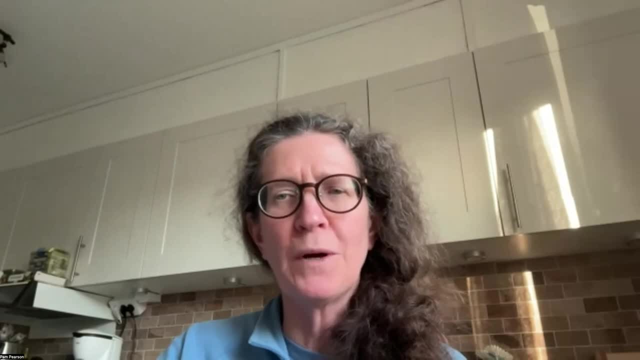 either in relation to IMO in the Arctic or to Antarctica. presentations.